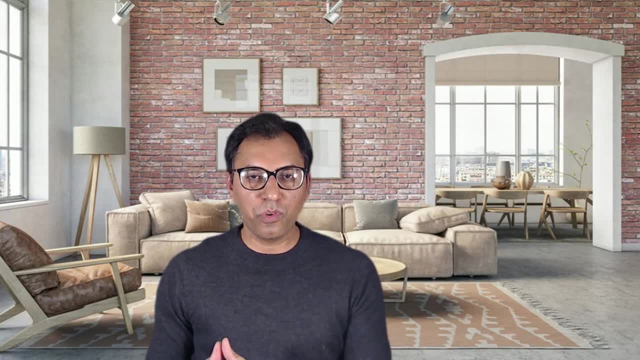 Hi everyone. This video is going to be really useful and informative because I'm going to explain full piping course in this video, Whatever the background you have- either you are in design, engineering, operation, maintenance, inspection or project management. This video is going to be really useful if you want to know about piping. It could be you are interested little bit about piping or you want to go in details. This video should be useful for you. 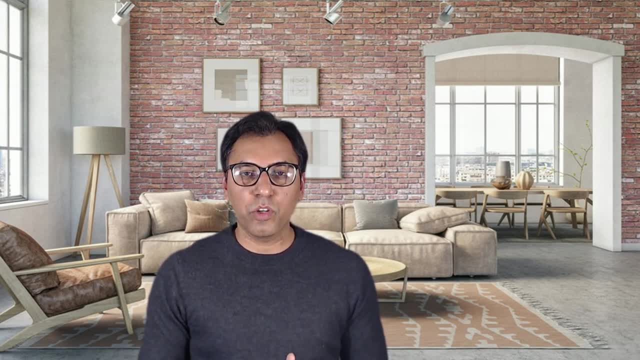 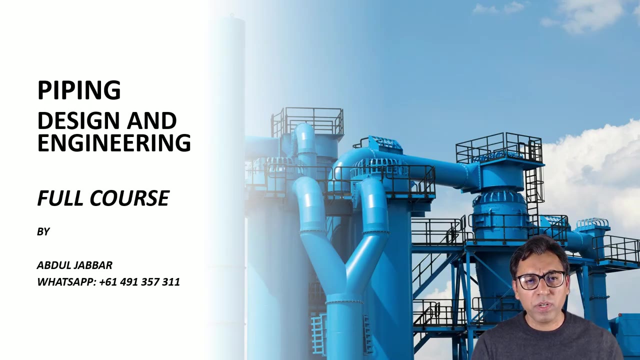 This video should be really helpful and I am confident this video will be one of the best videos you have ever watched about piping And this course in this video will be about one hour long video And, if you are ready, let's start. Just briefly about my introduction: My name is Abdul Jabbar and I have engineering background with over about 20 years of experience in different industries. 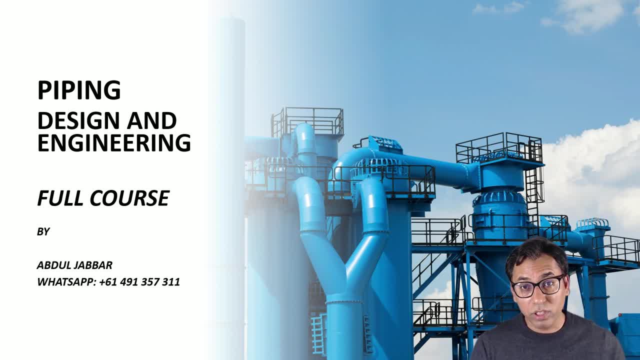 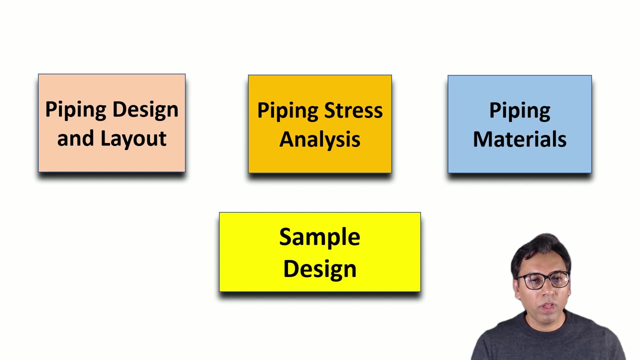 In hydrocarbon, petrochemical and process industries. I have performed multiple roles, and mainly my role was around piping engineering. All right, Without further ado, let's start piping design complete course. Broadly, I have divided this piping course into three categories. 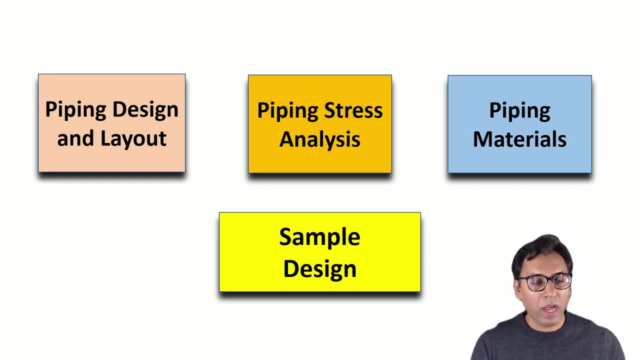 First one is a piping design and layout, And second is a piping stress analysis. Third is a piping materials. I will explain all these three categories first briefly. Then I will explain all these three categories with the help of a practical sample design of a plant piping. 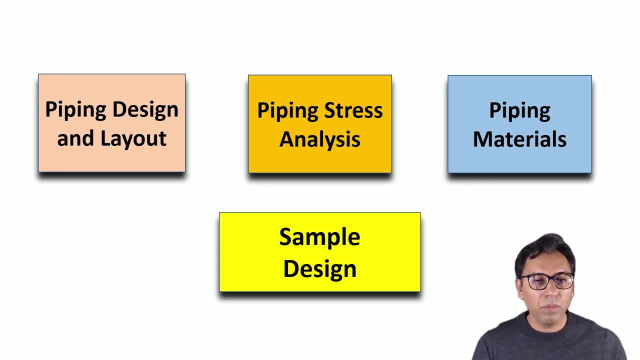 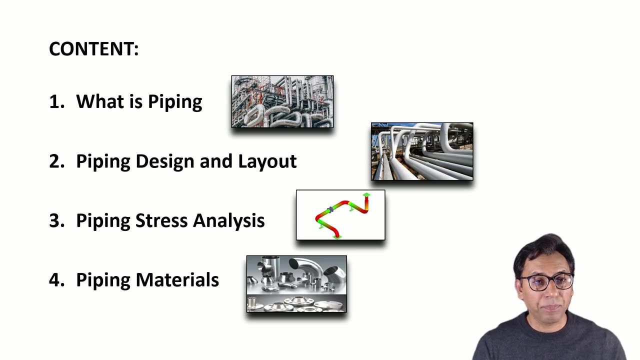 Let's first see what will be the core parameters content in this course. so the contents of this course will be. I will talk about first what is piping. it's a definition. then what is piping? design and layout, piping stress analysis and then piping materials, as I just briefly mentioned in. 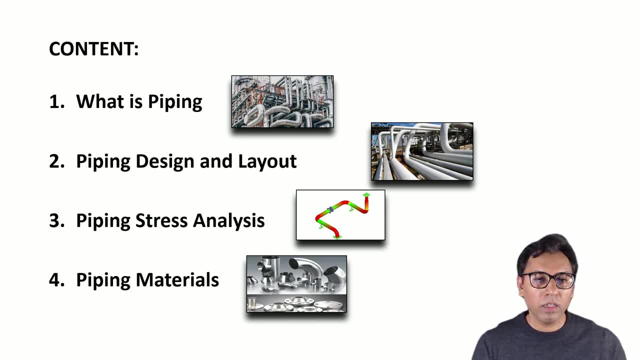 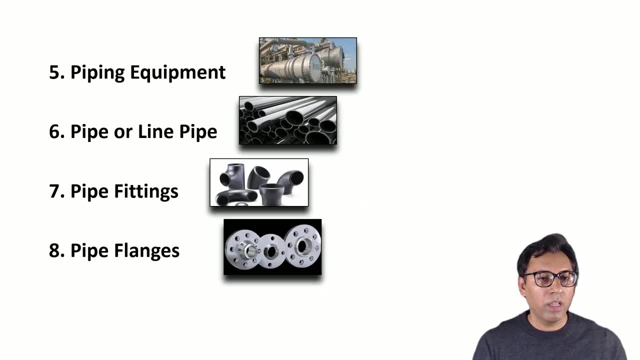 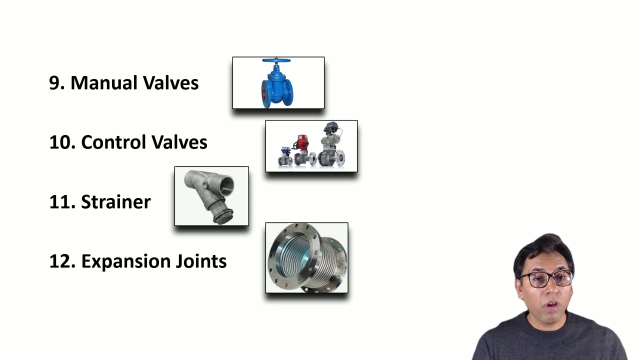 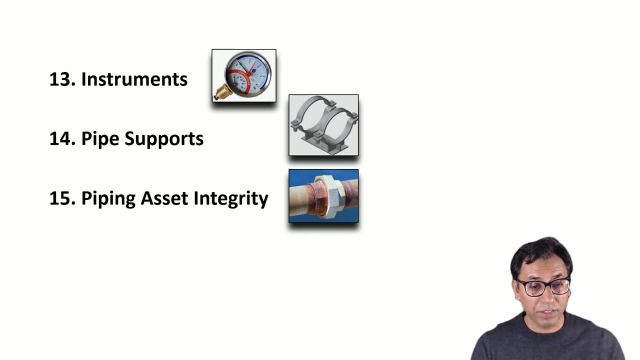 my last slide, then afterward I will use a practical example and explain all the bits of piping system, like piping equipment, pipe and line pipe, pipe fittings and pipe flanges. this practical example will show how to use manual valve, control valves, strainer and expansion joints. I will also explain about instruments, pipe supports in piping, asset integrity. 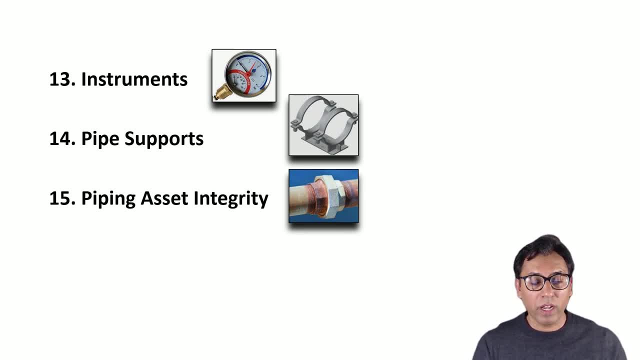 so you can see there are 15 contents in this course, one more. there is a timeline of all these contents in the description of your videos, so you can also go there and watch any content, whichever you like most or if you want to go back and watch. 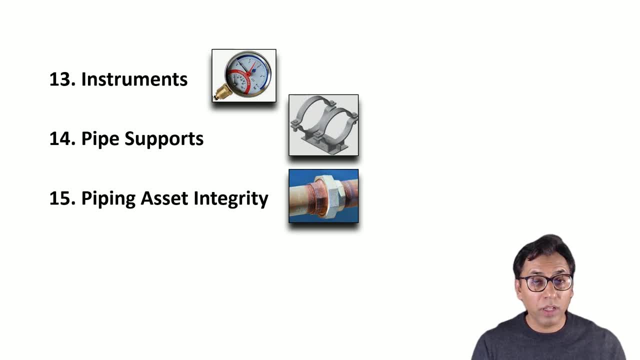 again that particular course. you can go there and watch that particular course content. you can easily go there. so all the timeline of this course is listed in this video's description. have a look at the description of this video if you have any question, query or feedback about this video about piping course and. 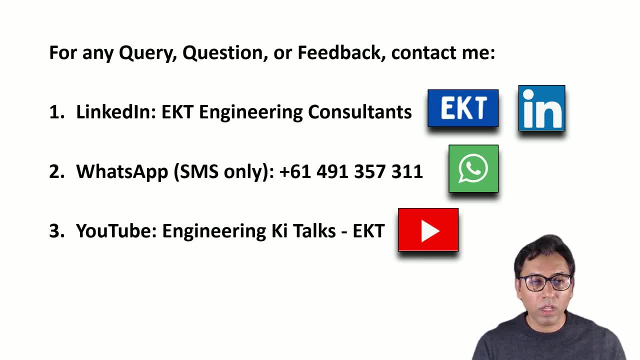 here is a contact details. you can follow me on my LinkedIn page. the address is a EKD engineering consultants. you can also approach me via whatsapp- only SMS, please, no call. also not necessarily about piping, but you can ask any question about other engineering disciplines as well, and even about job career. I will try to guide you as much as possible. 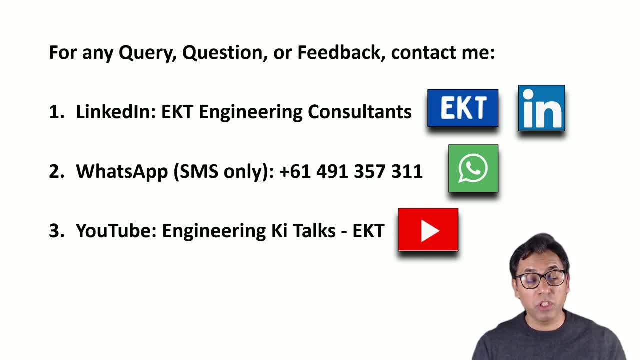 thirdly, if you want, you can also subscribe this YouTube channel. this channel will be one stop shop like and to get all the relevant knowledge, answer of your question, tips and about piping system. so I will see you in the next video. bye, bye. pipe engineering and other disciplines as well, also things I will try to share based 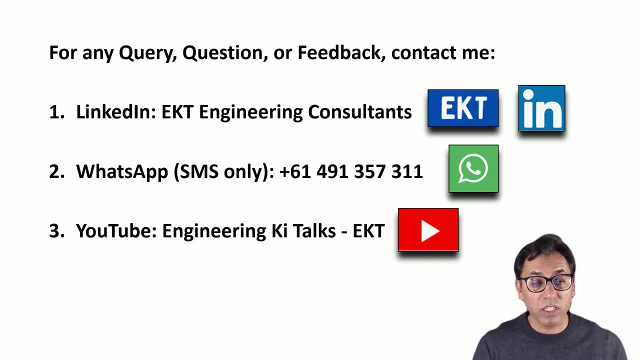 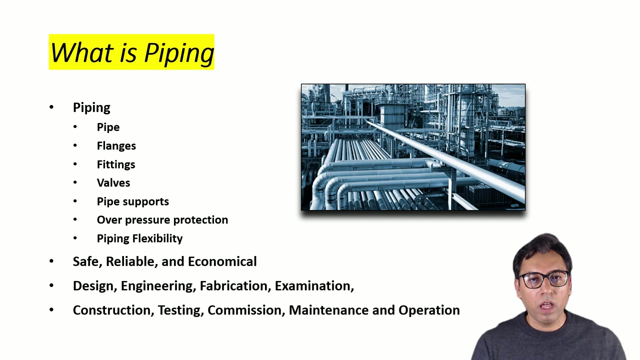 on my experience, knowledge and best industry practices. you can comment like this video. I will try to upload one or two videos in a week, not necessarily about piping, but could be other engineering disciplines as well. right, so first let's talk about what is piping. there are many definitions of piping, but 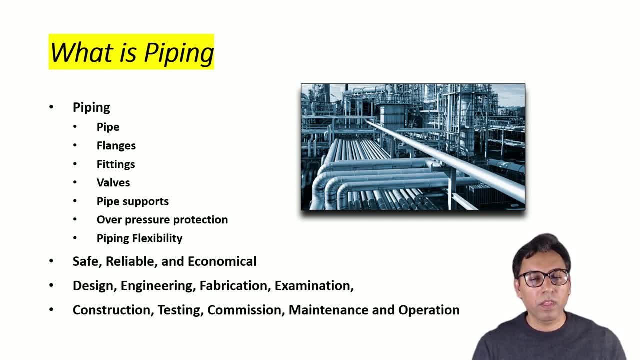 to cover all piping includes pipe flanges, fittings, bolting valves and pressure containing equipment could be special piping item. it also includes pipe sports and other items to prevent like over pressurizing and over stressing pipe sections when joined with fittings, flanges, valves and other mechanical 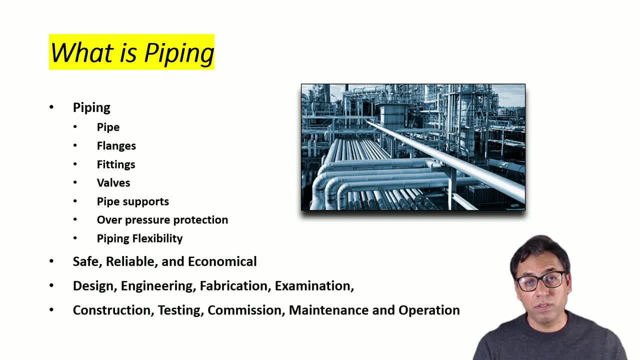 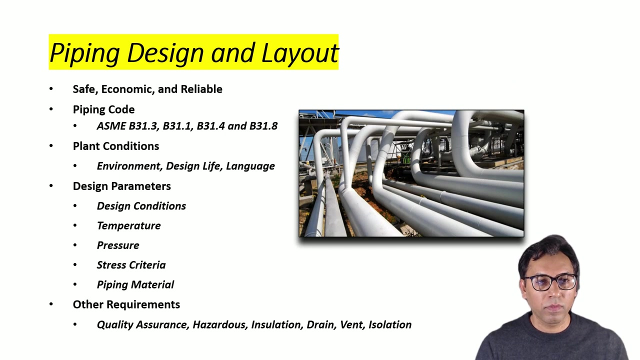 equipment and properly sported, they are called piping system- is safe, reliable and economical. piping system needs a good design engineering. it also needs fabrication, inspection, testing, commissioning, maintenance and even operation. now let's first talk about what is a piping: design and layout. it takes a lot of 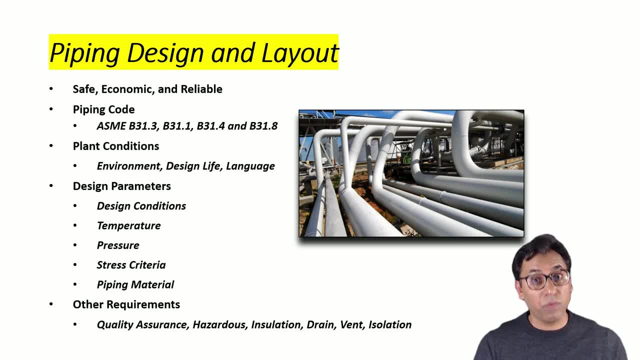 consideration, experience, knowledge, implementation of knowledge, experience and best industry practices to produce safe, economical and reliable piping system. I will talk about some typical aspects which need to cover to make this happen. first of all, to design any piping layout particular, first of all we need to decide what is a piping code which should follow local inclined needs and 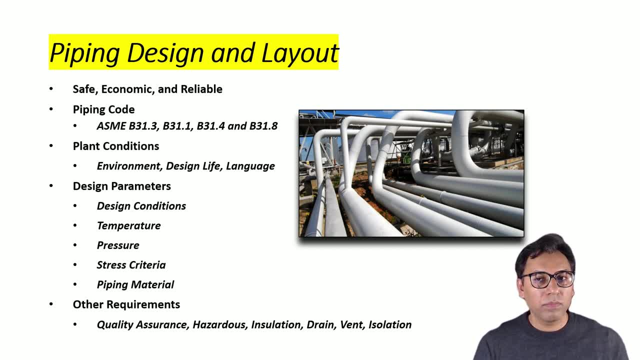 their expectations. for example, as me, be thirty one point three, process piping code, which is most commonly used code for a party. there could be other piping codes, like be thirty one point one, for power piping, and for pipelines we use b 31.4 or b 31.8, or could be other as well, depending. 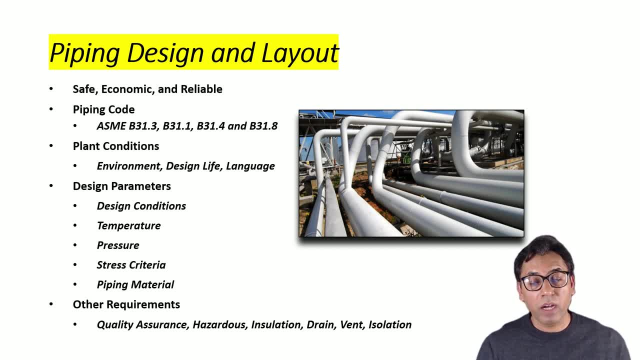 on which area, location or country that piping or pipeline project is going on. then we need to think about a general plant conditions like environmental conditions, plant design, expected life and what language we will use in design and drawings which will produce under piping design system. then comes to understanding design parameters for piping system. these may include: 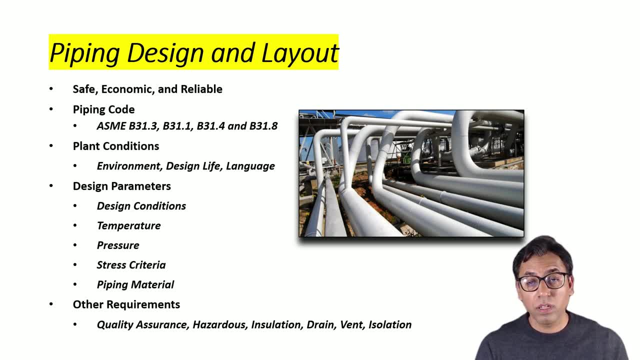 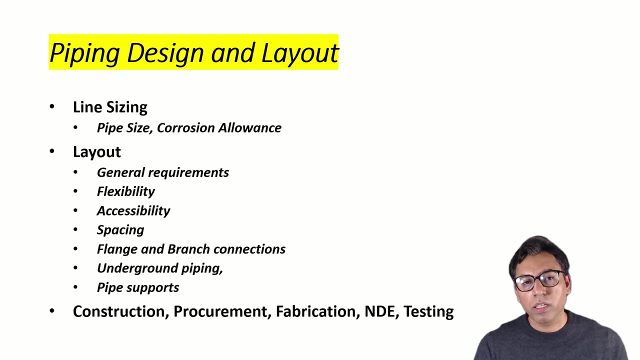 but not limited, like design conditions, operating conditions, pressure, temperature, stress criteria, piping materials, quality assurance, hazardous substances, insulation, drain and renting and isolation requirements. there are other aspects as well which we need to consider for a good piping design. they are like line sizing. it will involve pipe size, corrosion allows, erosion allows, depending on the type of the. 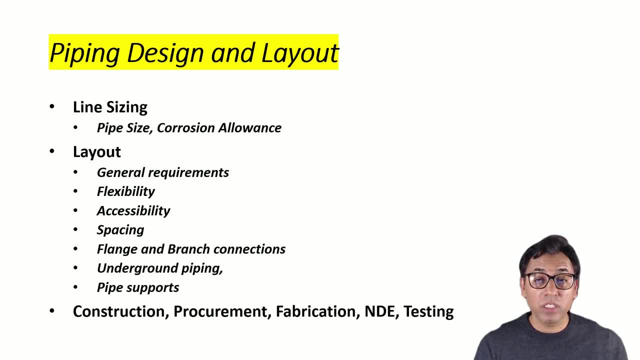 service inside the piping system: line velocities, piping layout. it will general layout requirements will be including, like piping flexibilities, piping spacing, accessibilities for maintenance, inspection, operation, flange connections and other connection details like pipe branches and it could be like underground piping pipe racks, pipe supports. so we need to 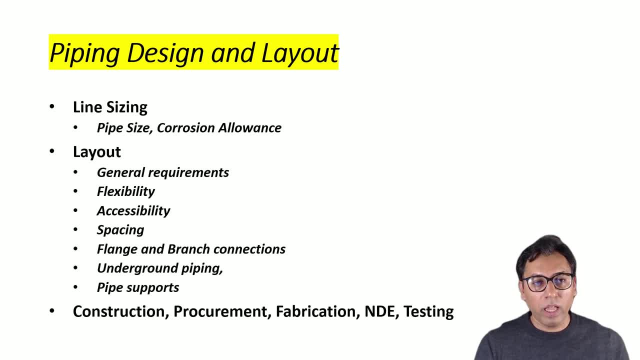 think about all these aspects and other aspects which we need to consider as well are construction point of view, procurement point of views, fabrication and NDE, inspection, testing and commissioning as well. one more thing: I have made a full video about feet, which is a front, and engineering and design. if you are interested, you can go. 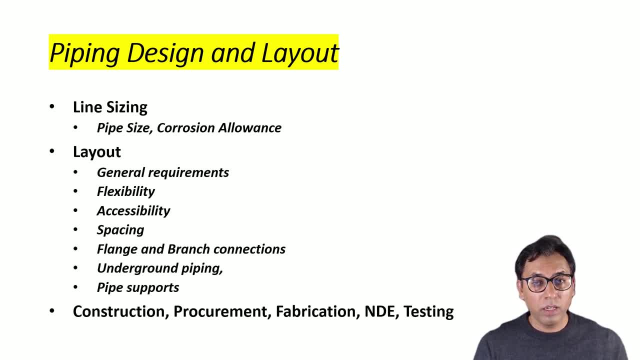 there and have a look, and link of this video is coming to top top right side of this video. you can click this or otherwise. you can go to this channel and there is a feed video which is going really popular and there is a lot of useful information about feet in there. 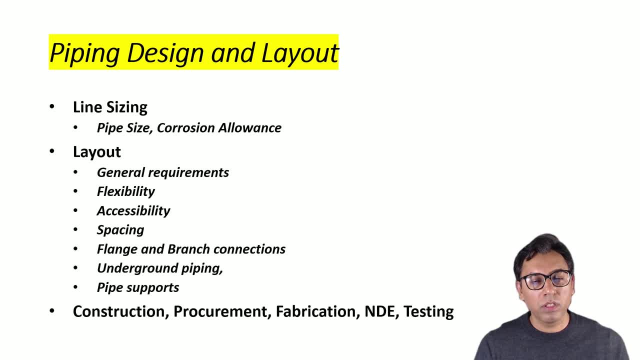 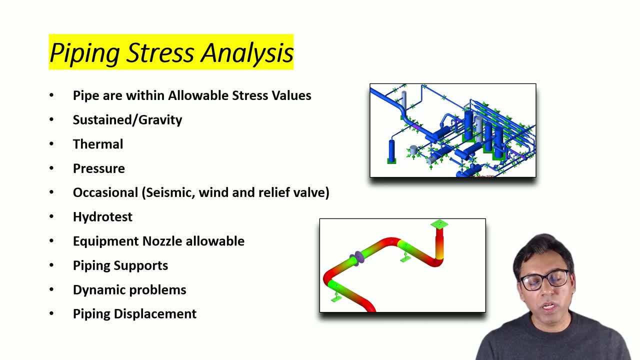 right now let's talk about briefly, piping stress analysis. whatever problem you have in your system, you need to know that. you need to know how to know how to do that. so the piping code we will use it could be b, 31.1, 31.3 or any. 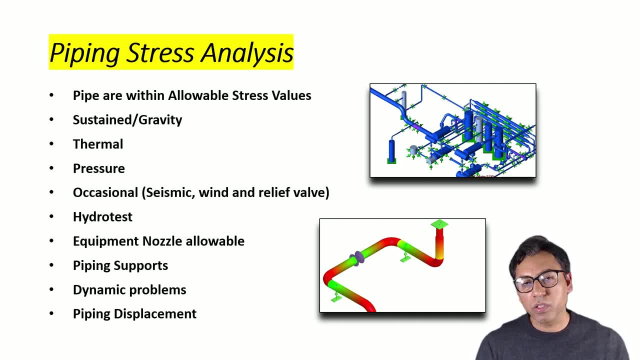 other code. it is a code requirement to make sure, whatever piping design we will do or we do, the layouting, the stresses produced in the system should be within the allowable of the code values. it's hard to cover full piping stress analysis details in a few slides, but I will try. 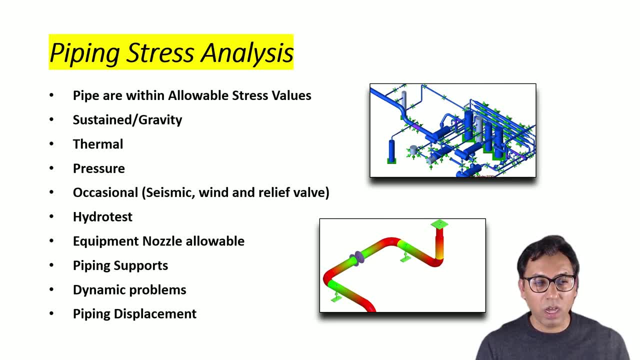 to cover the main highlights at least, I will talk about first what are the stress analysis objectives, inputs for stress analysis and what are the outputs for stress analysis. in this slide I will talk about what are the objective of piping stress analysis. stress analysis is required to make sure, as I said, 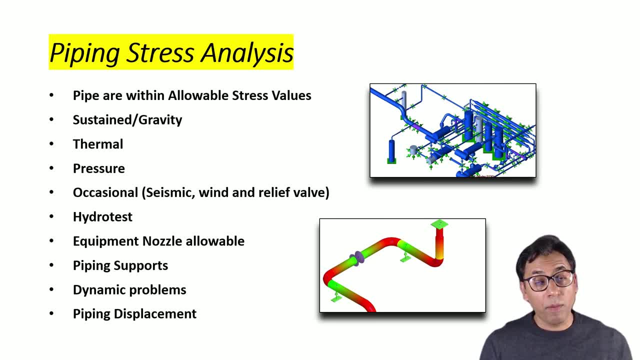 earlier to make sure all pipe- and it's what are the objective of piping stress analysis. it requires to be within the allowable stress range used under different stress categories, and these stress categories are: sustained or gravity pressure, thermal, occasional and high to test category for piping connected with equipment does not put 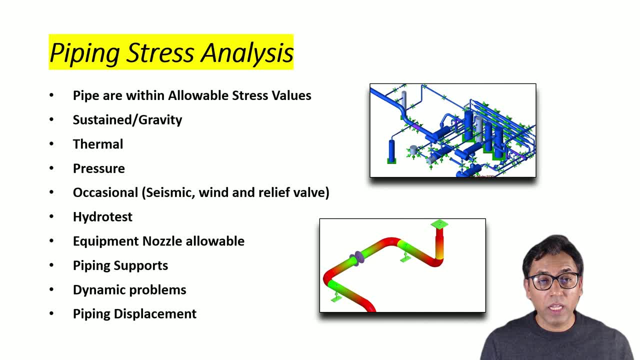 more loan than the nozzle allowable of that. that pipe supports and the load on those supports. and we also need to look after the dynamic potential problems. we need to check the pipe displacements. these are the main objectives to perform stress analysis and now in the next slide I will talk about what are the typical inputs to perform piping stress. 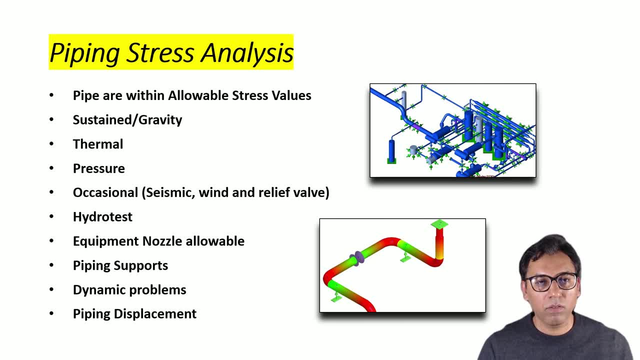 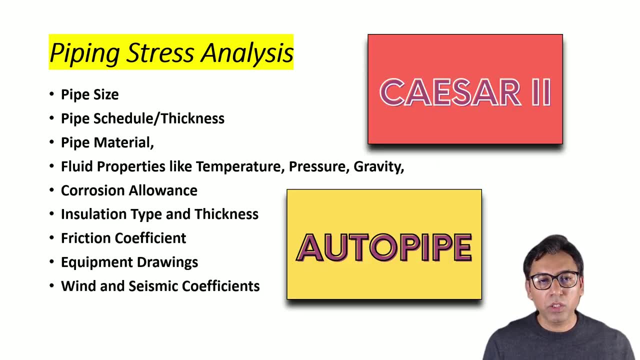 analysis. right, let's talk about what are the typical inputs for piping stress analysis. the two main softwares which we use commonly in industry for stress analysis are Caesar and Autopipe. the main inputs required for stress analysis are like: we need to know about pipe size, pipe thickness, schedule. we need to know 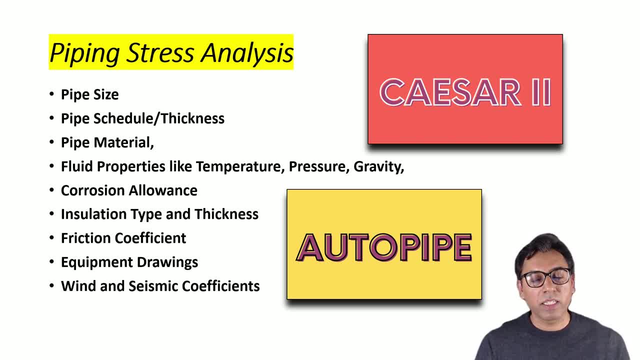 about pipe material flow properties like temperature, pressure, gravity, what is the corrosion allowance and insulation type, insulation thickness? we need to know what is the friction coefficient, equipment drawings, wind and seismic coefficients. so these are the typical inputs needed to perform stress analysis. again, this is just briefly and 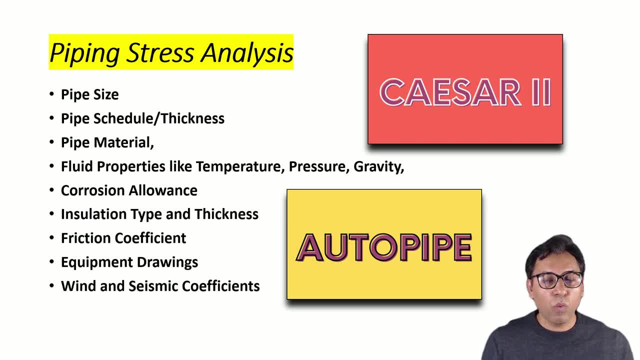 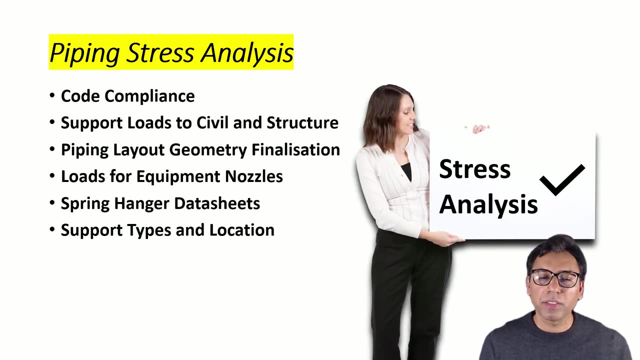 in next slide I will talk about what are the typical outputs of piping stress analysis. all right, now let's talk about what are the typical outputs of piping stress analysis. the main piping outputs are like to make sure the piping system which we design is a code compliant. 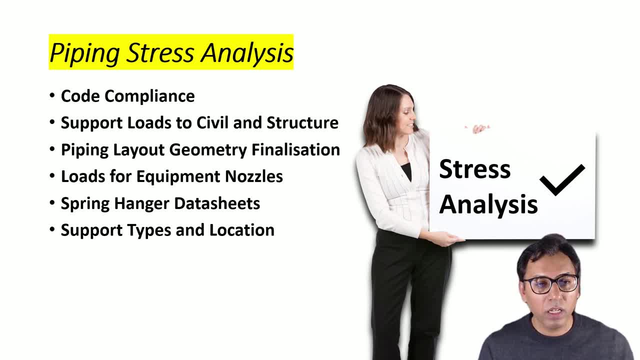 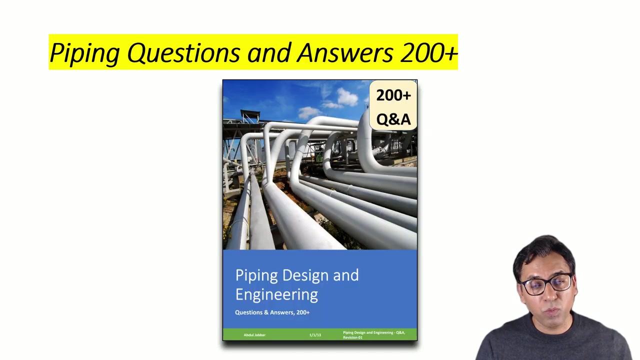 support loads for civil and structure design, piping layout, geometry, finalization. we will make sure the piping loads on the nozzles are within the allowable nozzle loads of the equipment and spring hanger data sheets. support type and location we do confirm after piping stress analysis right before going further. so just to summarize, 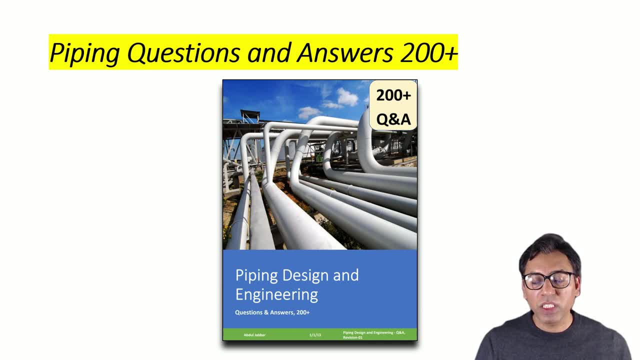 to, however, what we have gone through. we talked about what is the piping? we talk about what is the typical piping design layout. we talk about piping stress in factors. so far, before going further, just want to share with you- I think this is score knowledge, or even hard. 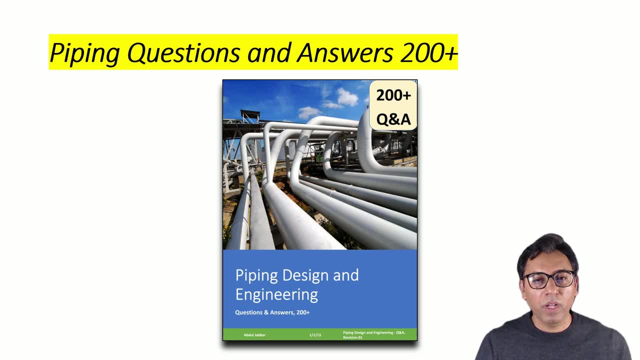 I'm super confident this book will improve a lot of your knowledge about piping because this is a practical questions, problems and their solution which I have observed over the period, my experience and all the content which I shared on LinkedIn or whatever I learned through performing a different type of 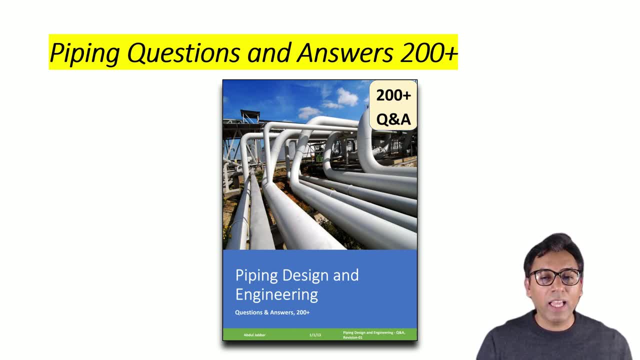 projects. this is a great way to understand about piping, as the answers are based on practical experience, knowledge, code, standards and best practice, rather than long theories just here. these questions cover all aspect of piping, like a design, material, stress analysis, code, fundamentals, and these questions can be used to prepare your next interview for job as well. and if 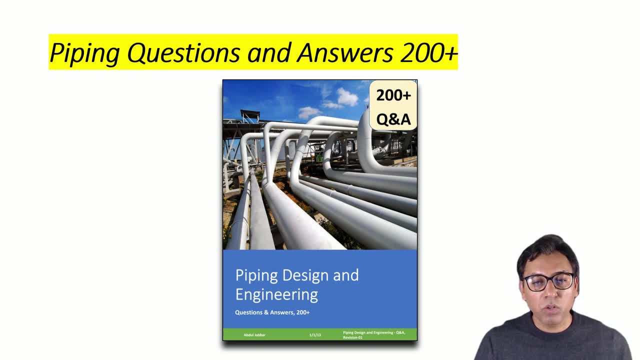 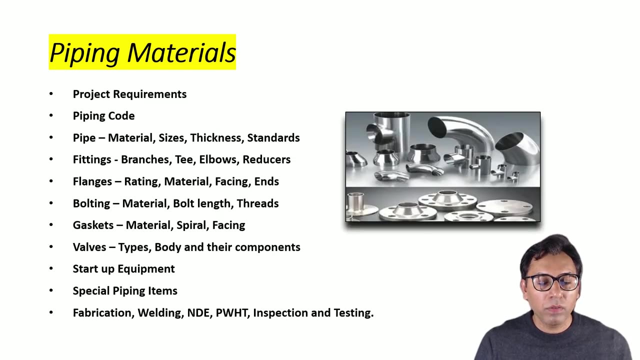 you are interested to get your copy, get in touch with me and to know more, and I will share the details from where you can get this book. all right, now let's talk about piping material, about. let's now let's talk about piping material for any project, or piping basically, any material of piping. 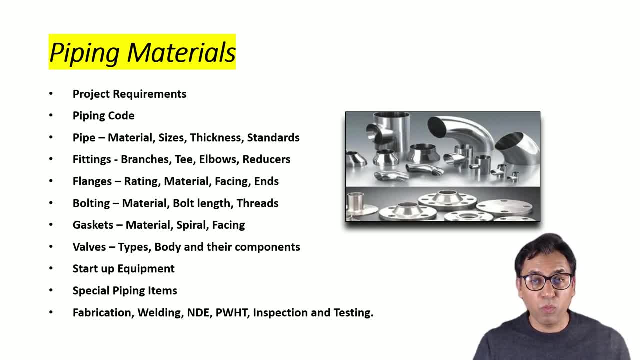 system is based on material selection criteria which we will make sure that that criterion meets the project requirements. also we need to make sure selected material meets that governing piping code because every code has their own approved materials. it's hard to cover again full piping material details in next few slide part. I will try to cover that. main highlights like 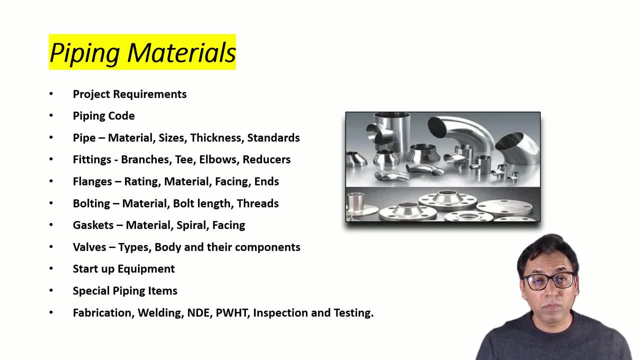 as an example of pipe. we need to understand what is the type of pipe needed for the job. it could be metallic, non-metallic, galvanized FRP, HDPE, stainless steel. Also, we need to do mention what will be the pipe size, what will be the schedule, thickness and for. 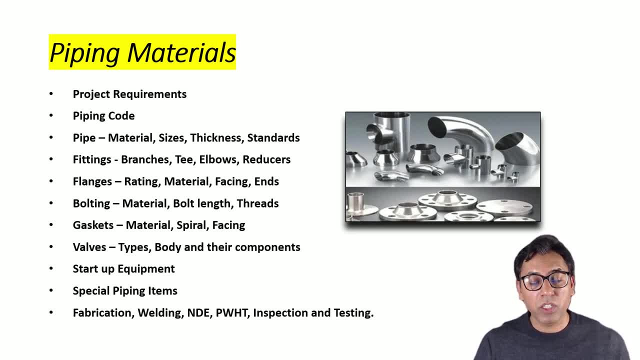 fitting standards, like we need to mention SB 16.9 or 16.11.. What is the required material, metallic or non-metallic? How about branches, tees, elbows and other fittings For flanges? we need to mention the required materials. 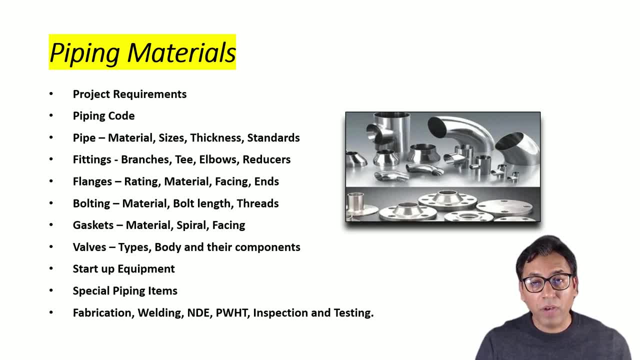 sizes, flange rating, flange facing and connection requirements. For bolting, what are the requirements of stud and bolt and bolt lengths required threads and also how about for gasket, Metallic, non-metallic, flat, spiral raised and other manufacturing? 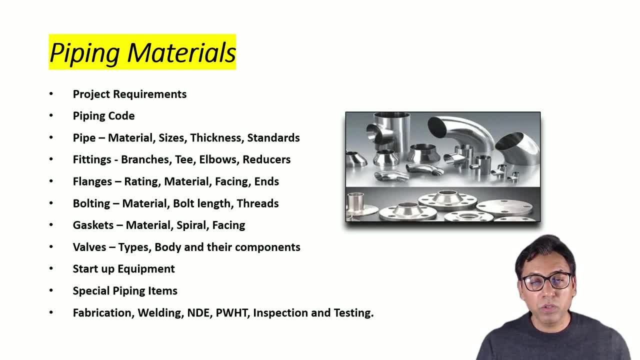 requirements For valves. also, we need to mention what will be the standard code type of valves requirement, including operation hand wheel actuator. do we need and what are the details about, valve body seat testing requirements, Then installation requirements as well. Requirement for special piping items, if 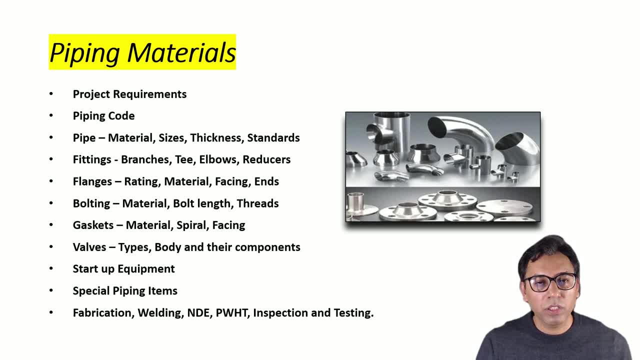 we use, and also they could be special piping items, like whenever start up of any new plant or after shutdown. we need, like startup strainers, temporary equipment, so we need to mention details about them as well. we also need to mention design, fabrication, welding, heat treatment. 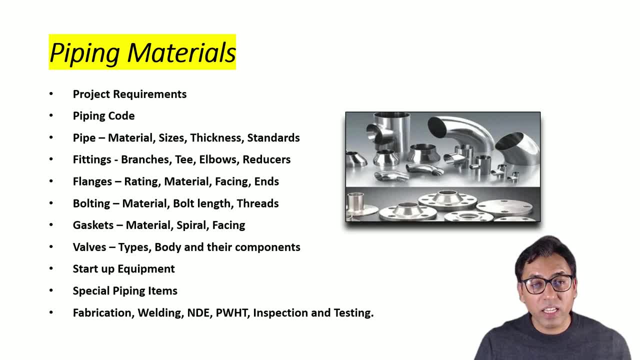 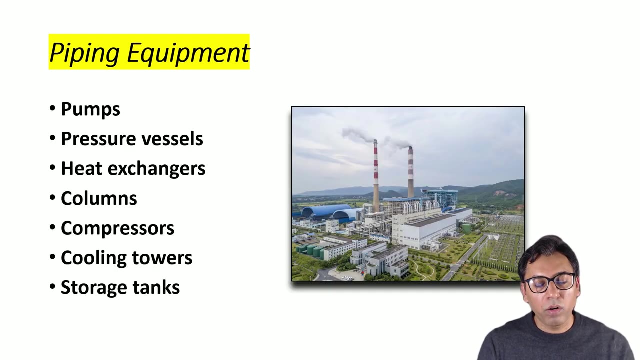 examination, inspection and testing standards as well. So basically we need t provide details, enough details of all these items as a minimum for any project material requirements. all right, so so far we have covered as a overview about the all three aspects of piping: piping design layout, stress analysis in piping material. now i will explain. 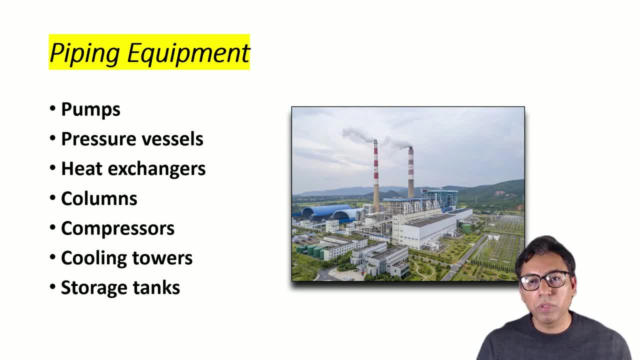 or whatever. so far we have gone through or learned through a sample design case of piping, so it should cover a lot of aspects and it should give a good explanation and and it should answer a lot of your questions. first thing first. let's talk about and understand quickly any plant refinery. 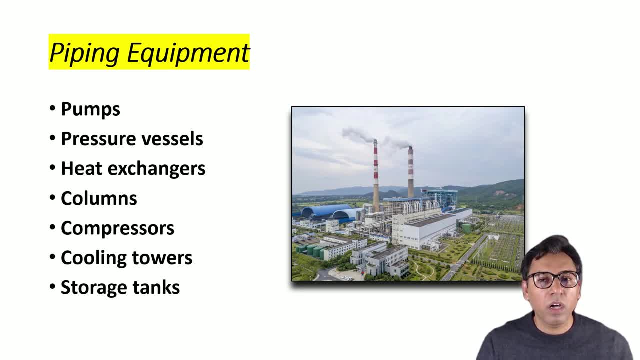 or processing facilities. there are range of equipments we can see in that facility. these equipments could be like pumps, pressure vessels, heat exchangers, columns, compressors, cooling towers, storage tanks etc. and all these equipments are connected with each other through piping here by role starts from popping point of view. we have interface with equipments like we need to know. 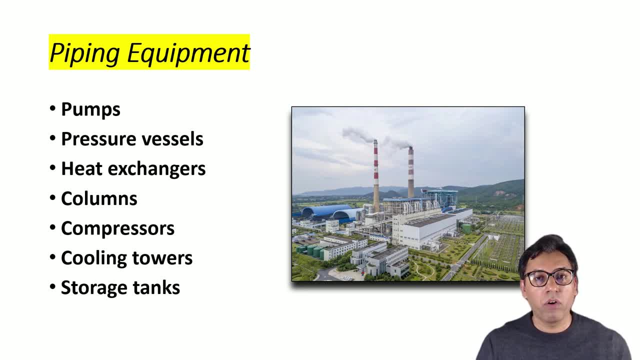 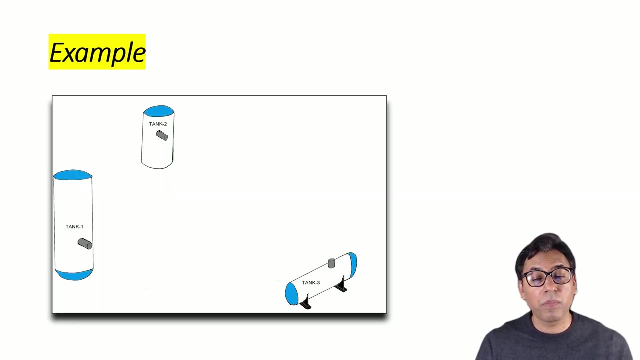 about their geometry, their orientation, nozzle locations, nozzle allowable loads, nozzle stressing details. all this information about pipe equipments we need to know because we will connect different equipments and here is the piping comes right. so for this video to understand about piping, i have taken as an example of tanks area. i will explain. 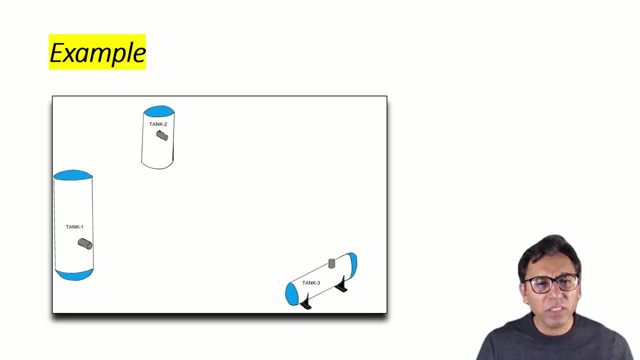 all piping aspects using this example. let's assume there are three tanks. these tanks have fluid inside and now we need to transport fluid from one tank to another, and one tank is a horizontal. I will keep referring this example again and again throughout my video to explain different concepts of piping, so hopefully this 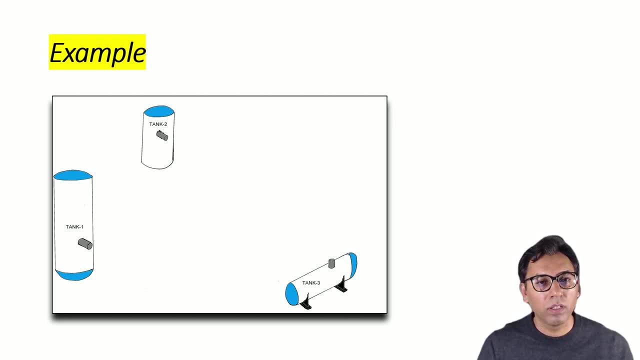 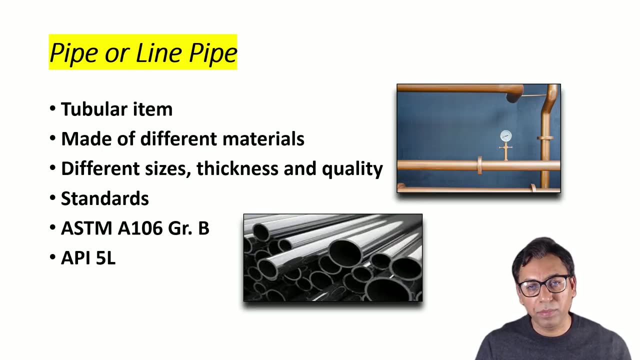 will be helpful for you. now let's first talk about pipe or line pipe first. for each equipment component, whatever, I will use example. first I will try to explain briefly and then I will choose that particular component of piping system in the example. okay, so first thing. first we will talk about what is pipe, what is a 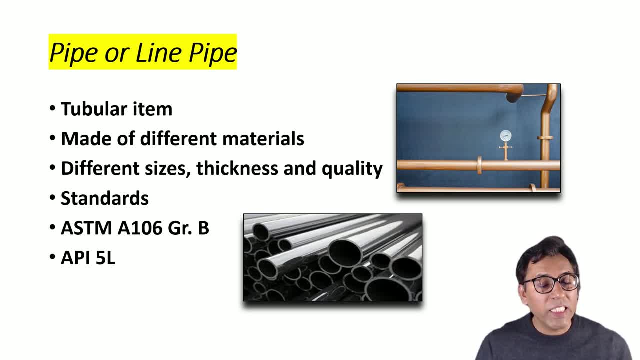 line pipe. what are the important details we should know? there are many definitions of pipe, but simple one is a. it's a tubular item made of material, including metal, plastic made for transporting liquid gas or anything that flows. it comes with different sizes, thickness and quality. there are 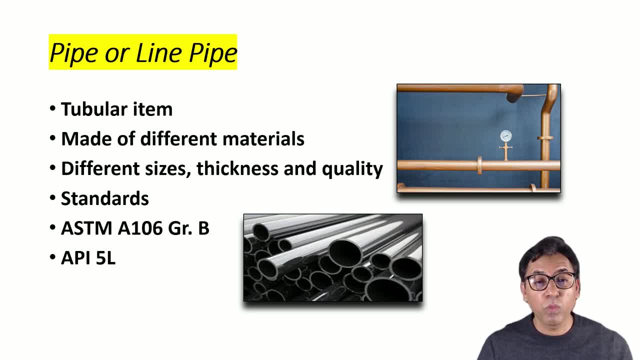 different standards of its manufacturing, but most common material for pipe is a ASTM A106 grade B for piping and if it's a pipeline, the most common material is a api 5l. if you want to know more about pipes, i have made a separate video about pipe as well. you can have a look. this and link is coming on top right side of this video. 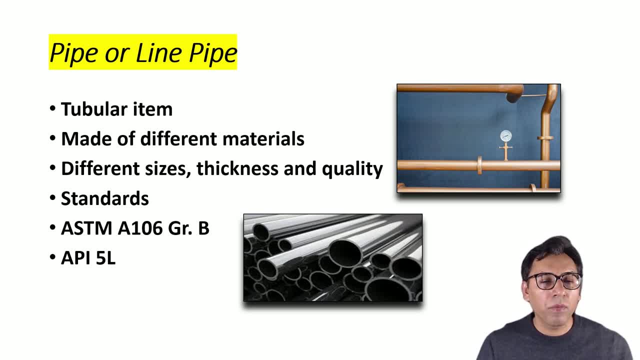 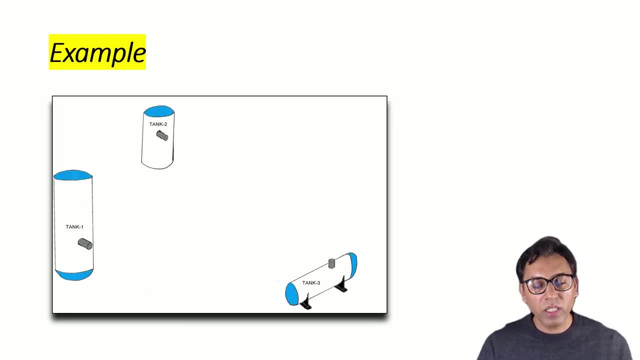 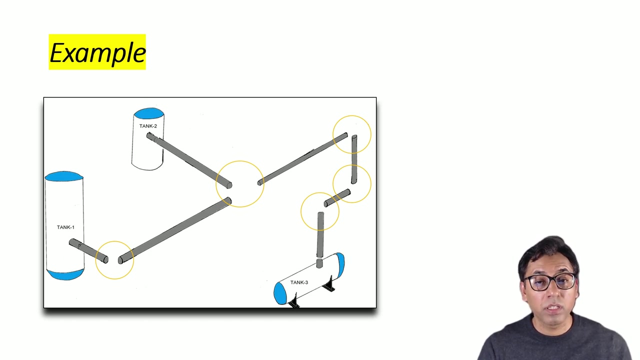 now let's bring back our example. we got three tanks. in order to transfer fluid from one tank to other, we need to connect them, so we will use pipes. alright, here we have installed pipes. you can see there are still some holes and free ends of pipes. these free ends will be fixed. 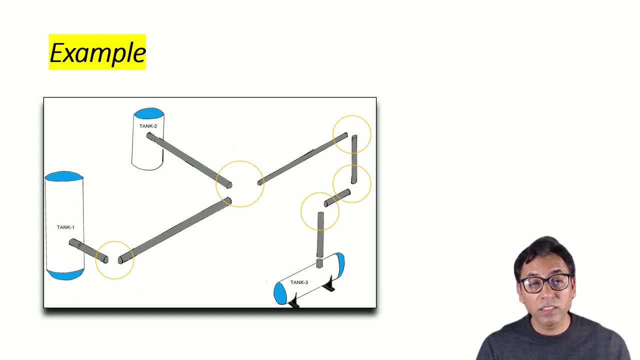 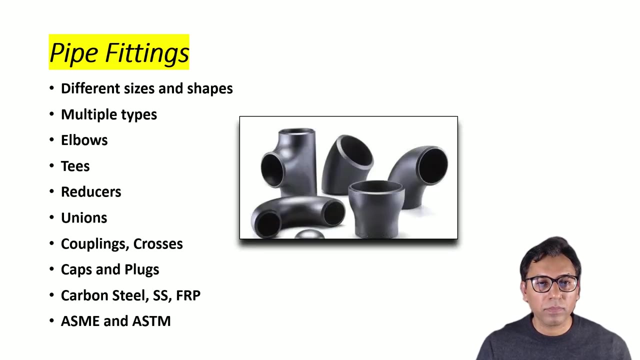 by pipe fittings. in next slides I will talk about how to address them as well. alright, before going further, let's talk about briefly about pipe fittings. Fittings are used in piping systems to connect straight sections of pipe or tube. They have different sizes and shapes. There are 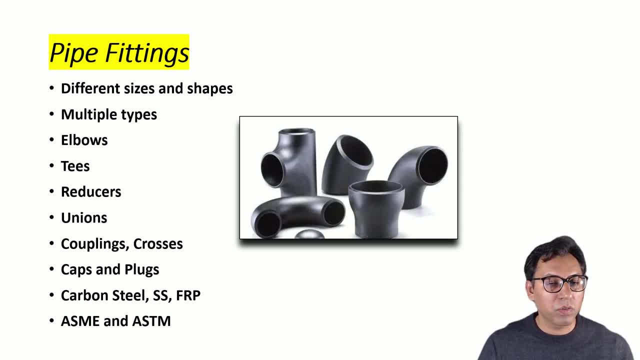 different types of fittings, like elbow tease, reducer, junions, coupling crosses, plugs as well. They are made of different materials, like could be carbon steel, stainless steel, FRP. They have ASME and ASTM and other standards of its. 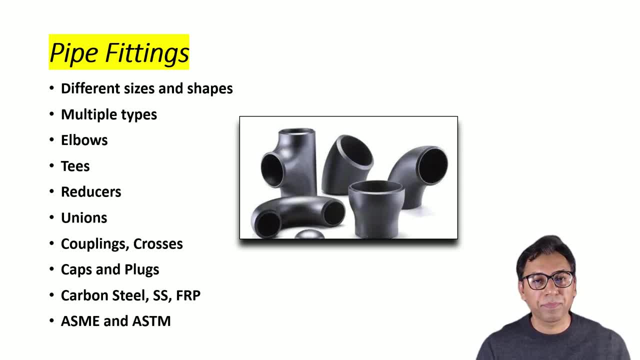 manufacturing. So that was a brief introduction about pipe fittings. Now let's use pipe fittings in our example and see how our piping look like. now We will use here 90 degree elbow equal T and reducer. So you can see we have successfully. 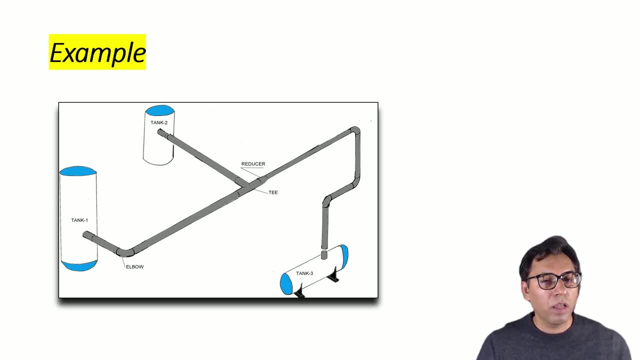 installed pipe fittings in our piping system is in a better shape now, If we can see here pipes are successfully connected. But in next step we need to connect piping ends with tank nozzles. these points we call terminal connections and we will use flanges and welding to connect pipe ends with nozzles of. 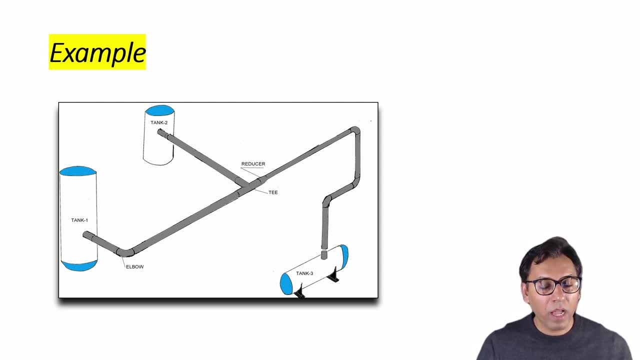 tanks. At this stage, pipe ends are not connected with the nozzles of tanks. those are free ends. we will connect them in next slides. first let's talk about pipe flanges, because we will use flanges to connect ends with a tank nozzles. a pipe flange connects. 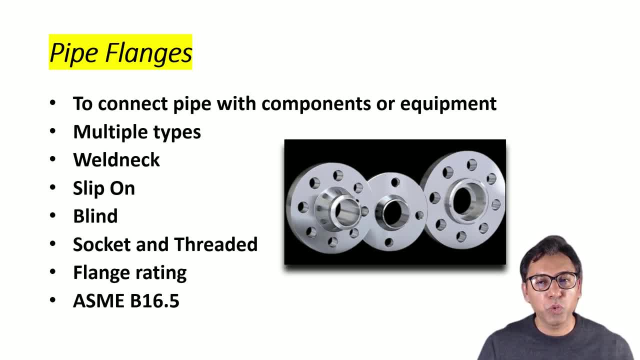 piping and its component in a piping system by the use of bolted connection, threaded or welding, and using gaskets. there are different types of flanges and some are, as example, well neck, slip-on, blind socket, weld and threaded. there are different classifications of flanges based on pressure and temperature in. 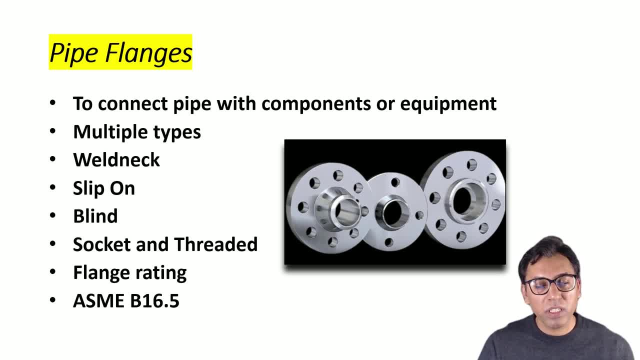 material, which we call flange reading. as me, 6d, 16.5 is the most common standard use for flange manufacturing. I have made a separate video about flanges as well if you want to know more about flanges and you can have a look and the link is coming at the top right side of. 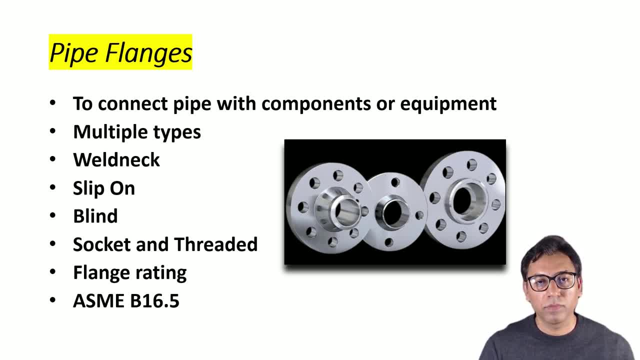 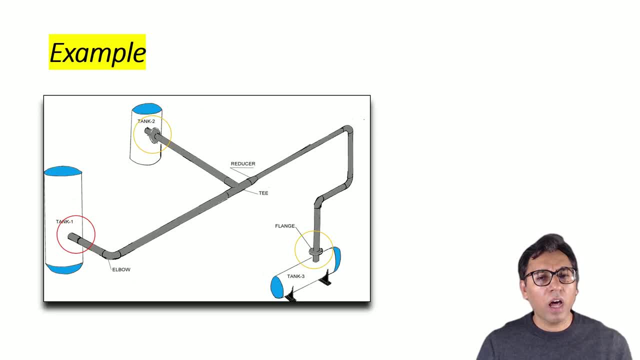 this video as well. now let's use flanges in our example and see how a pipe system look like. now we have used two flanges in this example and shown in the circle, so Tank 1 and Tank 2 or, sorry, Tank 2 and tank 3 have been. 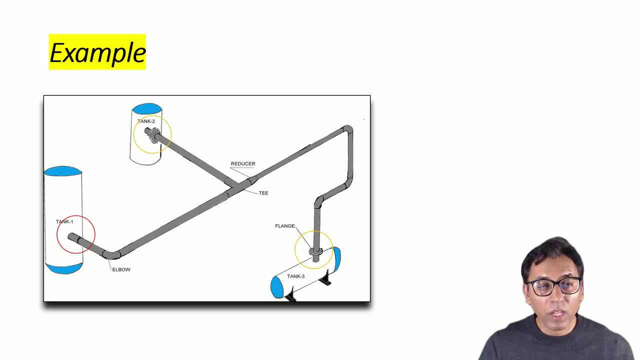 connected with the help of flanges. in the third tank, which is a tank 1, and in a red circle nozzle is connected with the pipe take over welding. so you can see now we have no loose end in the piping system system. we have used all basic piping components but there are many parts of the successful safe. 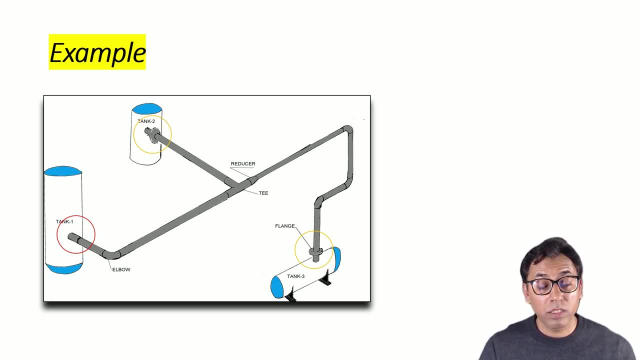 economical and reliable practical piping system still missing, which we need to cover in next slides as well. so far, if you have any question, query your feedback, do let me know and you can share, in the description of this video or other content, details which i have shared earlier. 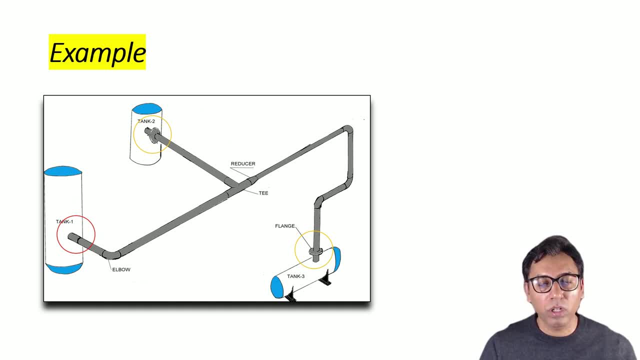 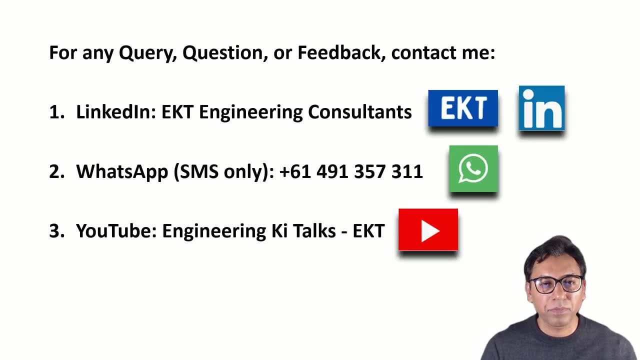 and i, just as a reminder, i can share in next slide as well. so these are my details: my linkedin page, my whatsapp number and again this youtube channel. now i will talk about first valves, because we have to use valves in our example as well. so let's talk about first what are the valves basically? 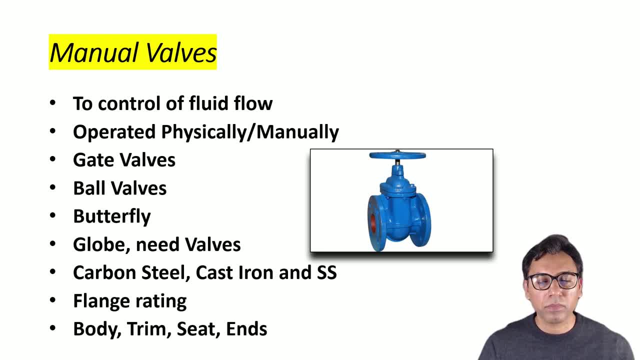 there are two broad types of valves: manual valves and control valves. valves are used to have control of load flow, to close, open or to regulate flow. in this slide, i will talk about manual valves. as name suggests, these valves are operated physically. there are different types of valves, like 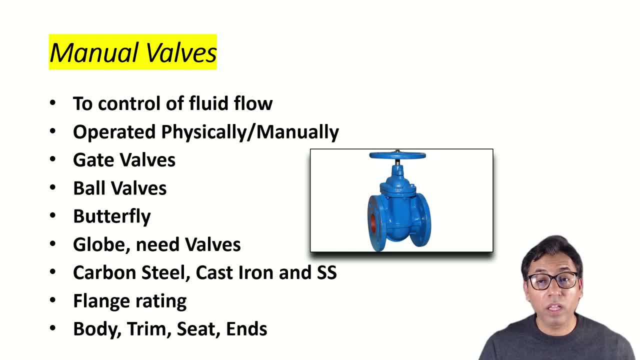 a gate valve, ball valve, check butterfly, globe, needle valve, etc. there are different construction materials like carbon steel, cast iron, stainless steel. they have different flange rating as well. they have a multiple parts like body, trim, seat and the valve ends as well. so we need to know. 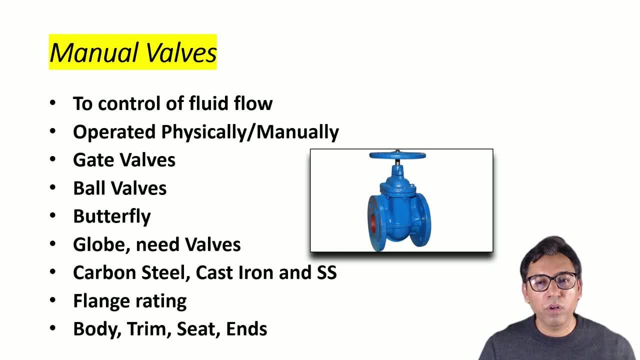 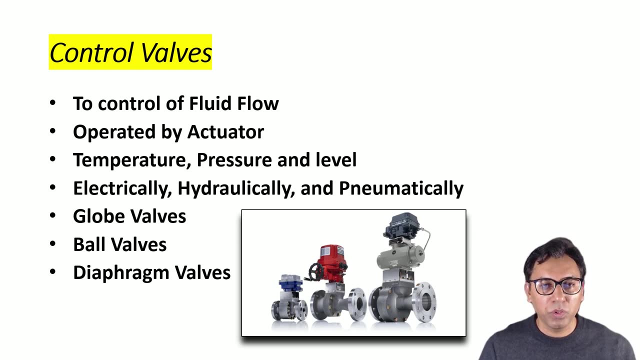 all these aspects of valves, especially whenever we will select well and we will go for procurement. now, in this slide, i will talk about control valves. control valves are used to control fluid with the help of signal from a controller or actuator. these valves are used to control the temperature, pressure, liquid level of the float these wells have. 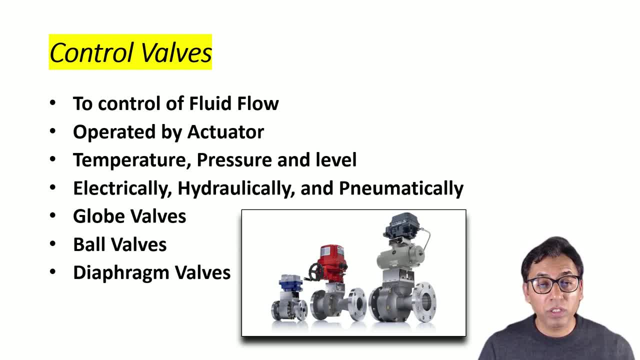 actuators and which are run by electrically, pneumatically or in amputation as well, so could be hydraulically. common types are glow well, ball well and like diaphragm valves. i have made a full video about valves as well, if you want to know about more about valves. 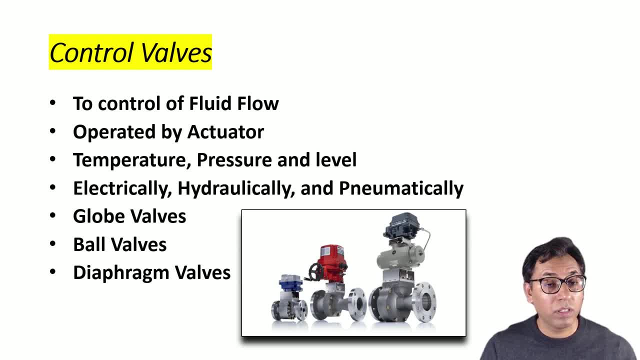 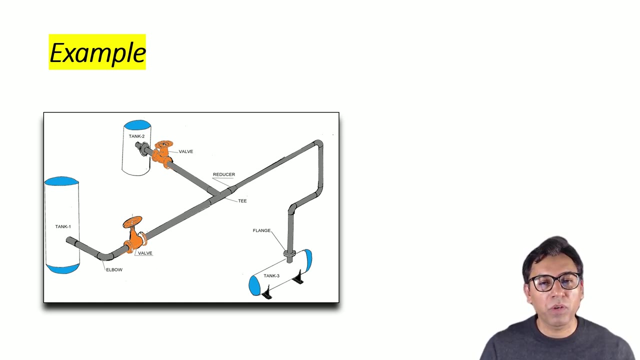 you can watch that video. there's a link of this video is coming to the top right side of this video. now let's use valves in our example and see how our piping system look like. you can see here we have used two manual valves. these wells can be used to control the fluid. 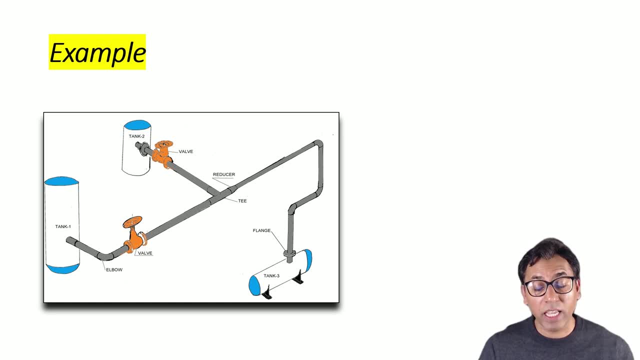 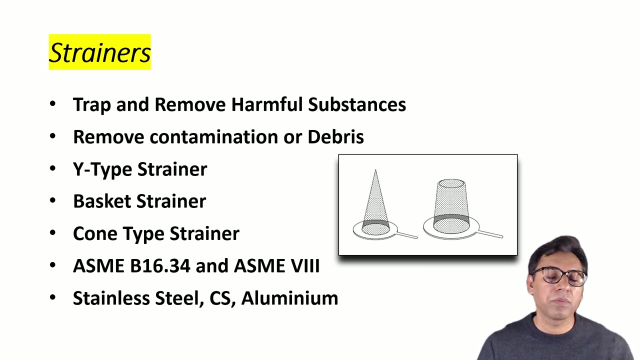 next thing which we will add here: in this example, a piping system is a filter or strainer. let's talk a little bit more about what is a strainer and then we will use that in our example. so basically, strainer is a small accessory or component that allows to remove and trap. 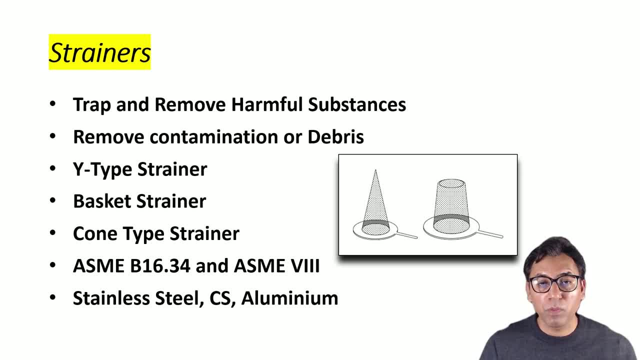 any harmful substances. strainers are used to remove any contamination or debris from the fluid which otherwise can damage the equipment like pumps, compressor, different types of strainers, like wire type strainer, basket type strain, some are temporary strainers as well and which we use like when we first start the plant. 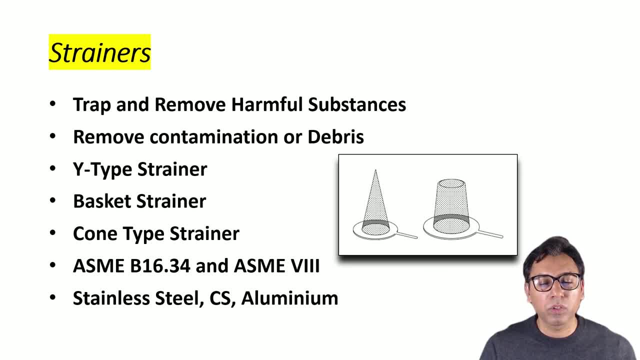 and during commissioning. most common standard use for strainer design is, as maybe or sometimes as me, section eight as well. they have different materials, but commonly stainless steel, carbon steel, and for mesh we use normally aluminium. Now let's use strainer in our piping design example and see how it look like now. 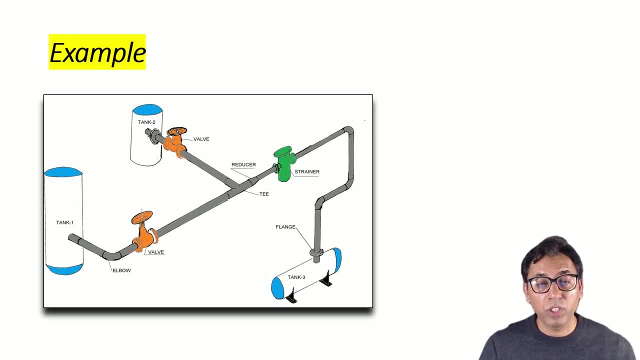 You can see, here we have used one strainer which is a basket type. This will help to remove any unwanted particle to go to tank 3.. Now we will add more elements which are also really important. So in next slides we will use expansion joint and this should give some flexibility to our 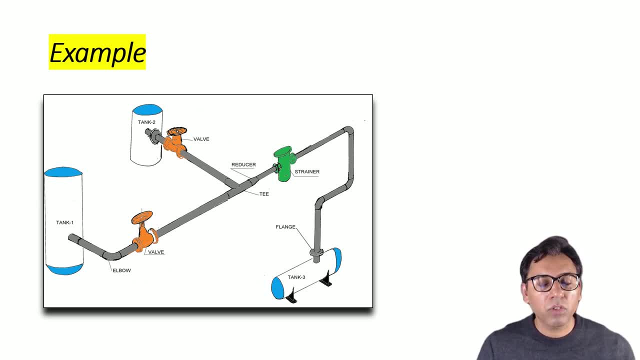 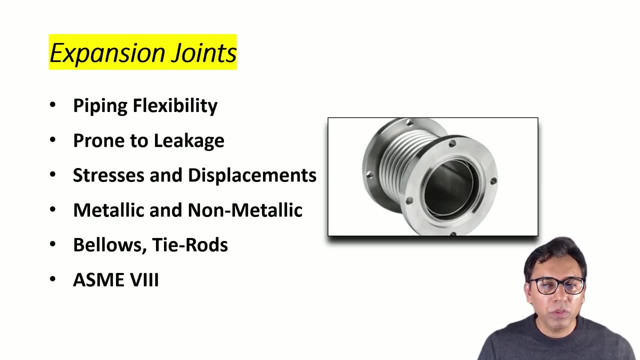 piping system. First, let's talk about what is an expansion joint. We use expansion joints as a part of our strategy to give flexibility to our piping system. We don't use expansion joints quite often as they are weak joints and they are prone to leakages. 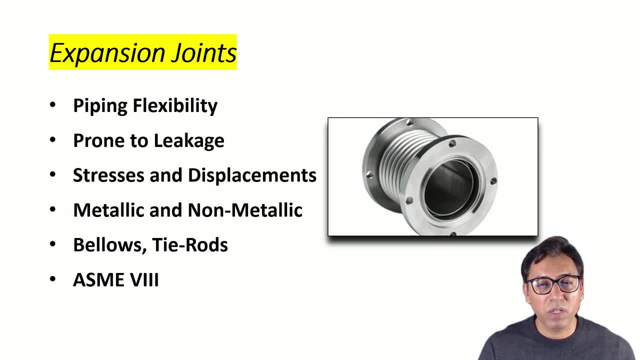 But if we have to accommodate piping, stresses, displacement, we provide expansion joints as well. The material can be metallic, non-metallic, depending upon the requirements. Common types are pillow or tie rod type and their manufacturing design standard commonly is ASME section 8.. 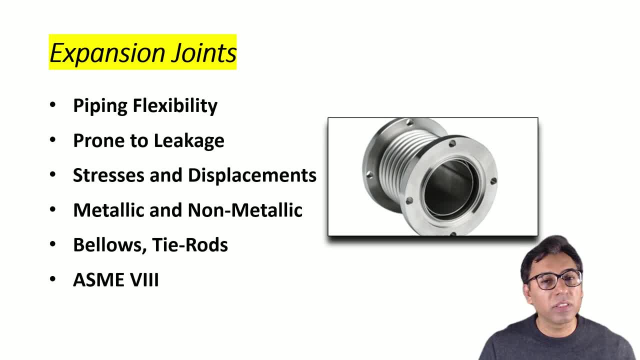 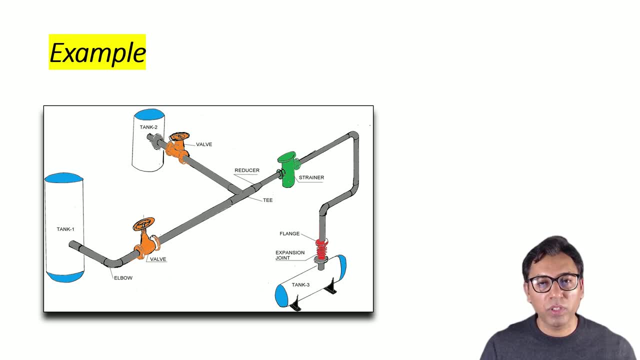 Now let's use expansion joint in our example and see how our piping system look like. You can see here we have used one expansion joint which is a bellow type. This will give flexibility to our piping, especially will manage load on tank nozzle. Now we will add some piping instruments to know about. 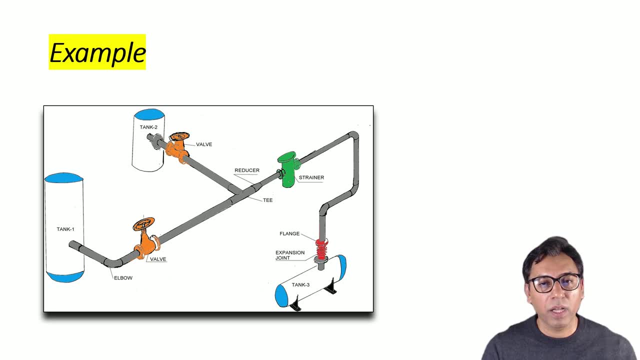 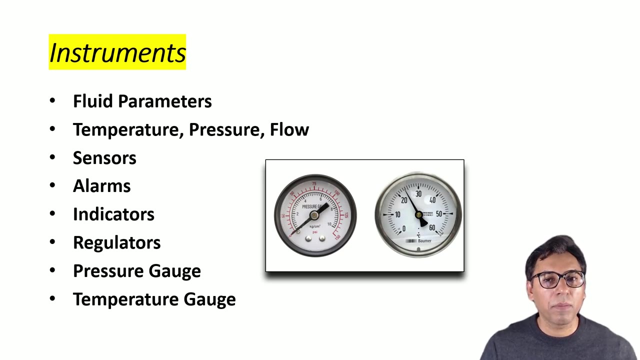 Now we will add some piping instruments to know about. First, let's talk about what are piping instruments. When some fluid is flowing in a pipe, we need to know about some parameters, including pressure, temperature of the fluid. To get that information, we need to install some elements which we call instruments. 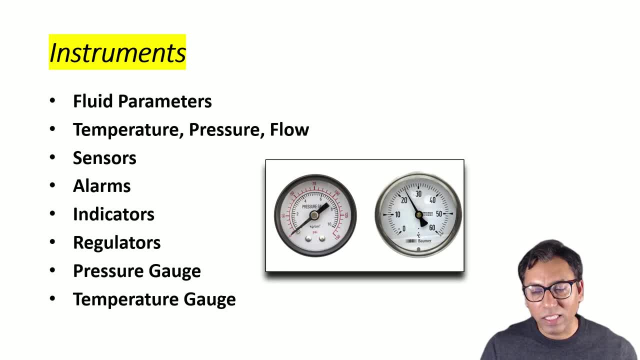 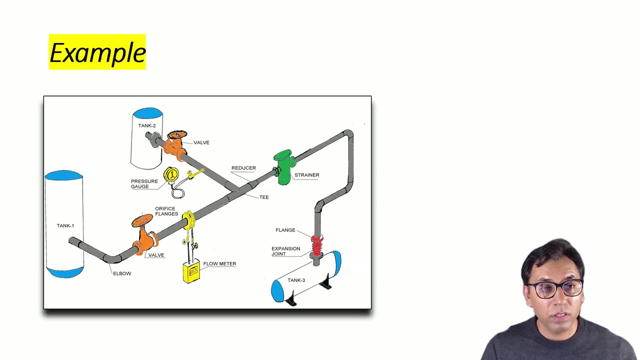 different types of instruments, including sensors, alarms, indicators, regulators, transmitter, pressure gauges and temperature indicators. Now let's use them in our example. You can see here we have used pressure gauge flow meter in this example. This will give us control to know different parameter of fluid. 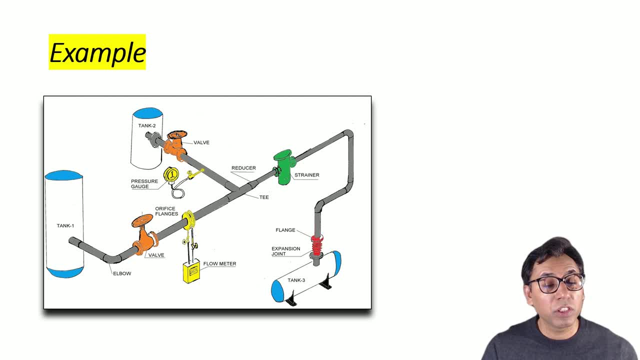 inside the piping and accordingly we can calibrate process conditions to meet our project objectives. Now we will add some piping supports. This will give safety and reliability to our piping system. First, before using them, first let's talk about and try to understand what are. 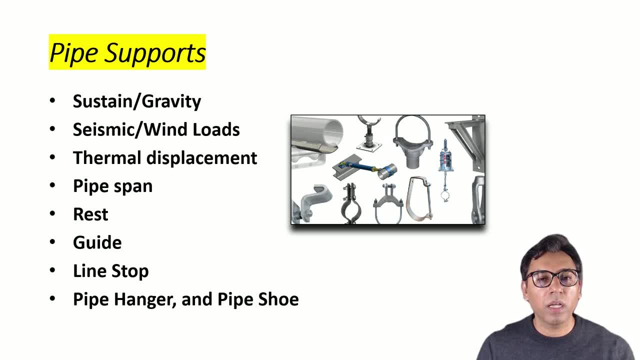 piping supports. We need different types of supports to give reliability to our piping systems due to different reasons. They are like for sustained or gravity case to give constraint for load and displacement, for seismic and wind case to manage pipe span, and it could be to 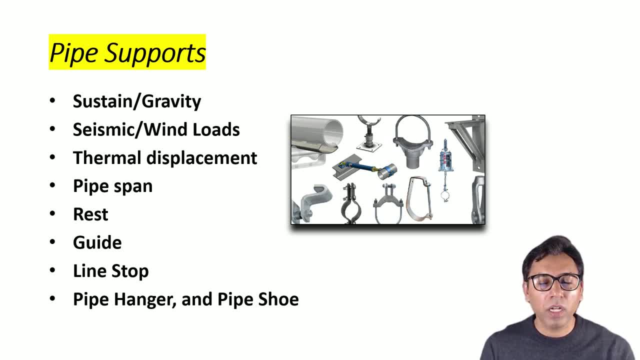 manage pipe thermal displacement. Common types are arrest or V type systems. Now let's look at some of the piping supports that we have used in our example. First of all, we have used some of the piping supports. We have used pipe hangers, pipe shoes and dummy leg and elbow. 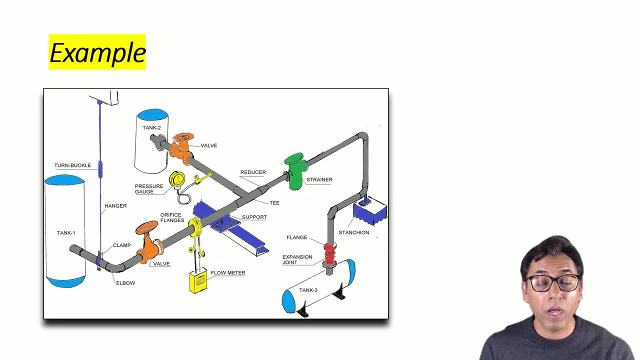 We have used pipe hangers, pipe shoes and dummy leg and elbow. These have given strength, constraints and flexibility to our piping system. After this piping layout, we need to do perform stress analysis, as I explained earlier in this video. Right Now, when we talk about piping and 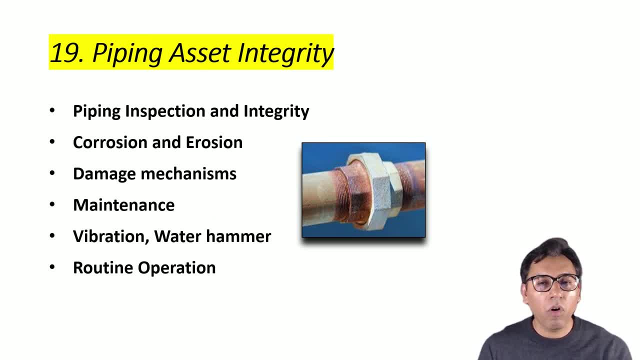 design and engineering. we need to think about all aspects of piping system, not only design or engineering, but also about the inspection as integrity maintenance in other aspects as well, because either that's piping system is designed for 20 years, 25 years, so it should be good for that particular. 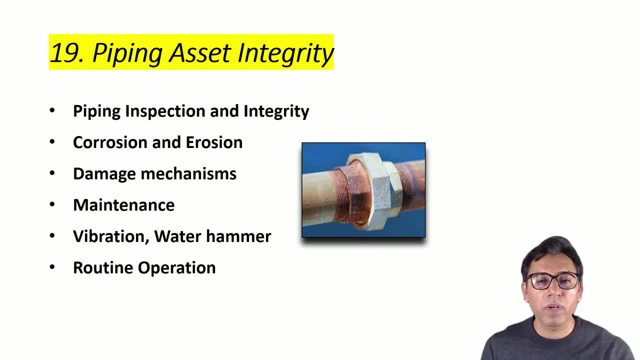 period and integrity requirements and common other inspection. operation problems are really important to consider as well. they could be like how piping can be saved or prevent from corrosion and erosion, what are common damage mechanism and what material we should select to cover those problems, damages and what is the type of the fluid. and it could be like the: 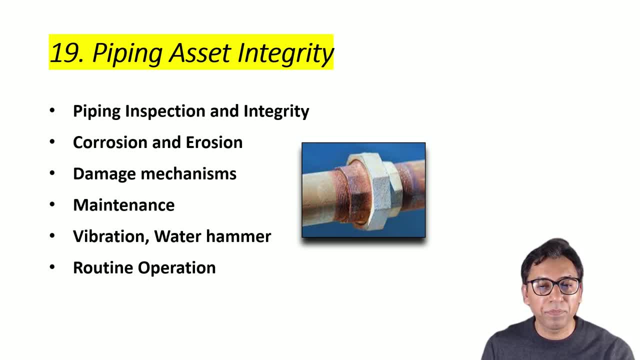 environmental impacts as well. so if it's a coastal area or the harsh environment, so that should also consider in the piping design. so our design should be compatible for maintenance and routine inspection and operation requirements. piping should be saved from the maintenance and the routine inspection and operation requirements. 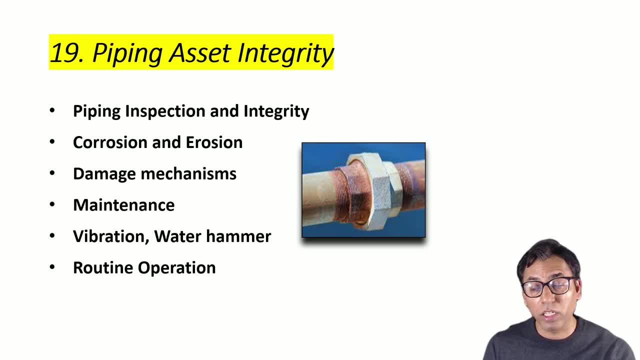 vibration and water hammer like issues as well, but we should be well placed to allow operation, sports activities and there should be enough accessibility for the people, equipments and, like the crane and other supports for the personnel. all right, piping course is almost over. I have covered all the aspects of piping. 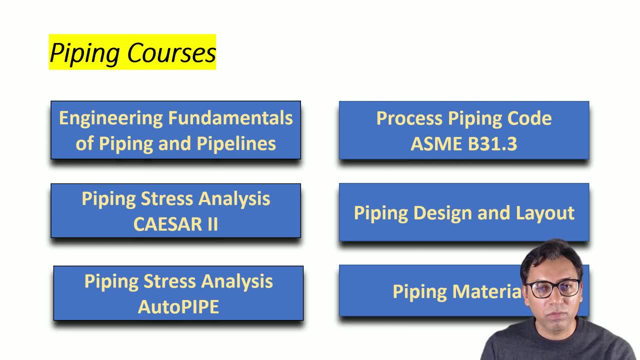 briefly again, that is just like tip of the iceberg, because the piping is a quite in-depth field, discipline, and it requires, in details, knowledge, and especially when you use that knowledge in any particular project. so it has to be compatible with the requirements and every project is different, so we have to use best practices, standards, course kinds of. 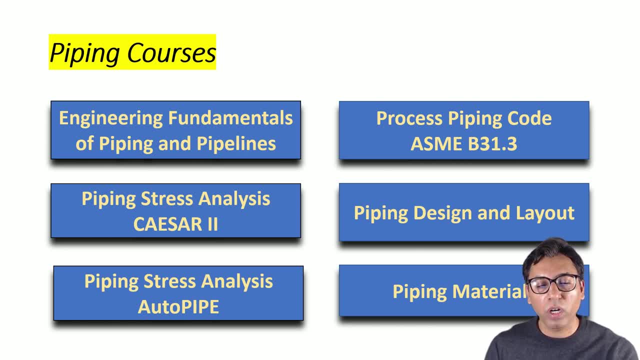 requirements and to make sure all aspects, whatever we propose in the piping system, starting from piping component, all the component mostly I covered in this course, so those has to be a compatible with the code standards. and and again after layout we have to make sure material and stress analysis. 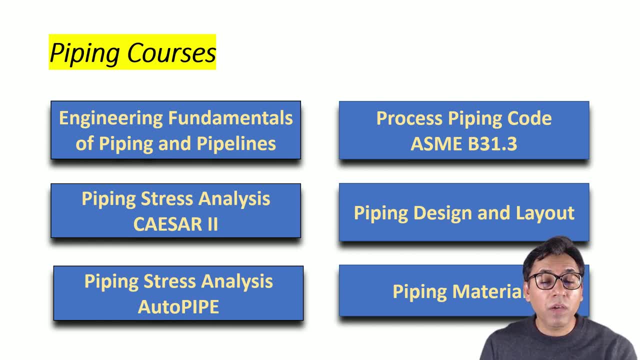 requirements are also met. I believe this has covered all the piping as well, but if you want to learn more about any area, I have these six courses as well which you should get if you want to enhance knowledge and confidence about piping. there's about. let's talk about briefly about these courses which I think we 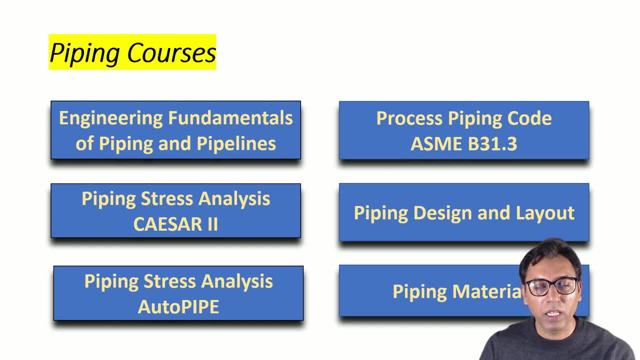 should cover all the critical aspects of piping basically in more details as well. I have already talked about the questions. you can get that one as well, and apart if you are interested to expand your knowledge, any particular area of piping. so so these courses might be helpful. so first one is a engineering fundamental of piping and 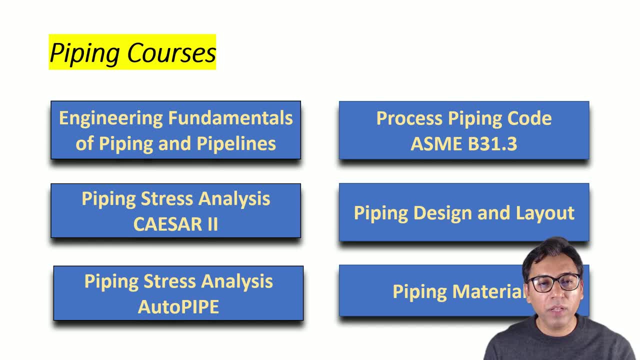 pipelines. so basically, this course covers all aspects of by VIM broadly. you can say: whatever you have watched in this video, this course will give you% $$$%theseäus number of components which would be at pプaring. we are going to provide more as we go further so you can discover about the vehicle materials in this�� 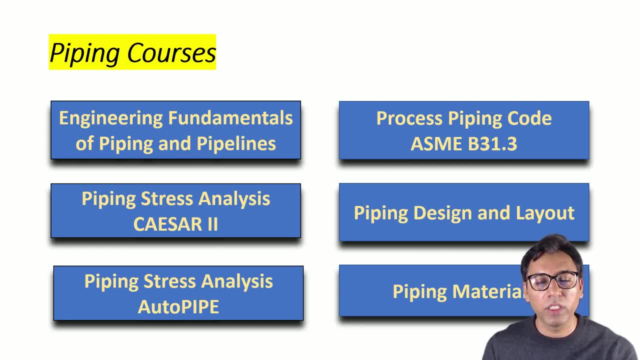 talk about in more details of all these aspects and with the more practical examples as well. this is very useful if you want to know overall piping basically. next is a piping stress analysis using freezer tool. this course is a very important and could be helpful for stress analysis. 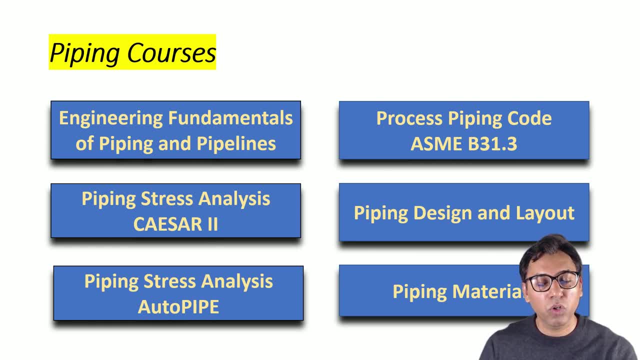 if you are interested about that and if you want to know about more like what are the fundamentals and the basis of stress analysis, with the reference of the codes and their inputs, outputs, how to stress analysis, use example concept principles, that course may be helpful. next is a piping stress analysis, but a bit about but using software autopipe. so basically this course. 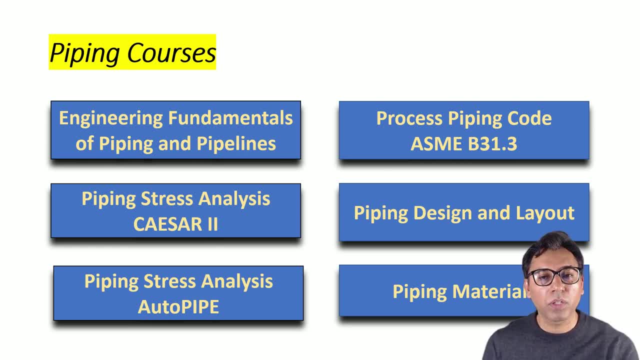 is also uh, covers most of the experts, as the previous stress analysis course, but the tool has been used different, which is auto pipe. next course is understanding and application of process piping code. as i said, as in b31.3, is the most commonly used uh course, so that course is. 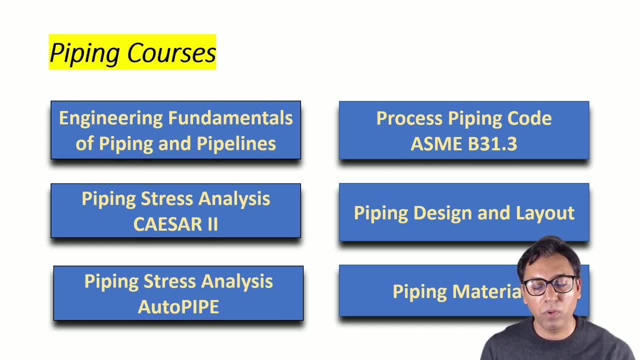 talk about all aspects, as maybe 31.3, starting from the design, starting from about the different components, requirements and the material, and talk about the fluid types and then the entity and structure. of course, this course is something i think we will go through. ah, the more and more. 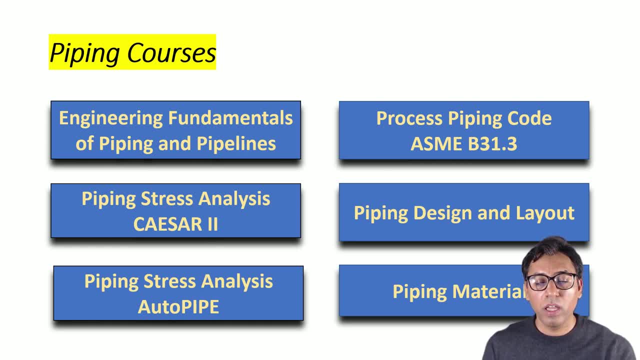 our- uh, the expectations for the course, and then to know more about the what is the purpose of the course and also that time frame. so that's how the course is handled. that's how to learn more about the process. then we will talk about the level of materials in the course, one of the things that 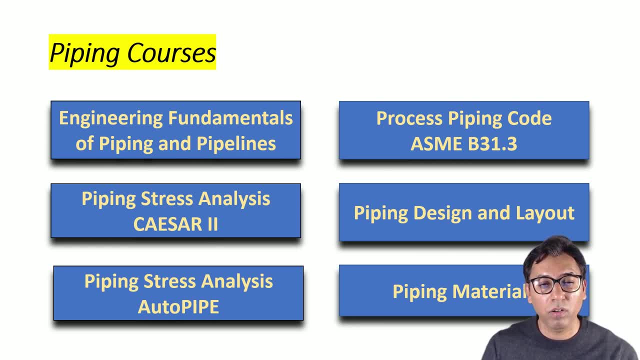 we try to show here is very important is the, the design of the design, so of the complex operation, but also the design of the port, the of the layout in the course. so, like i said, just touch base, just briefly, what should be considered in the piping design and 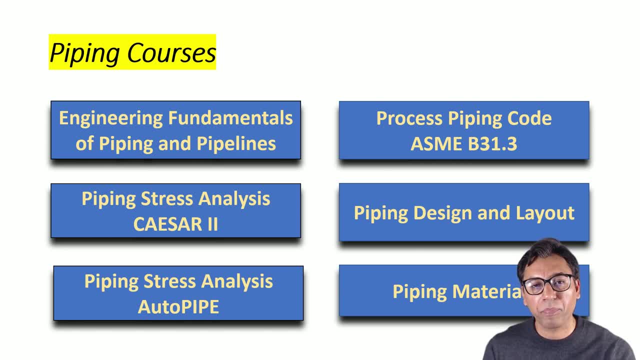 layout, but there is a lot of things when you do piping design layout up and like, for example, if you have to do a piping design around pumps or around the columns, they are so many aspects you need to consider and this, this course, will include aspects of design, engineering and best practices, and 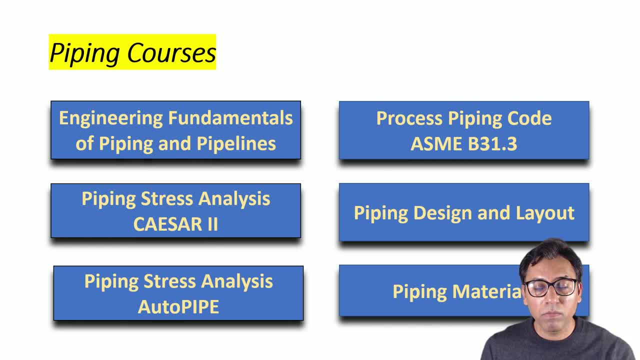 standard codes, references, and it could be like piping rack heat exchangers and, as I said. so there are best practices like: how about the like, the producers and fittings and the supports, what should be the support and what should be the supports? we know there are so many fittings and the pipe supports and what 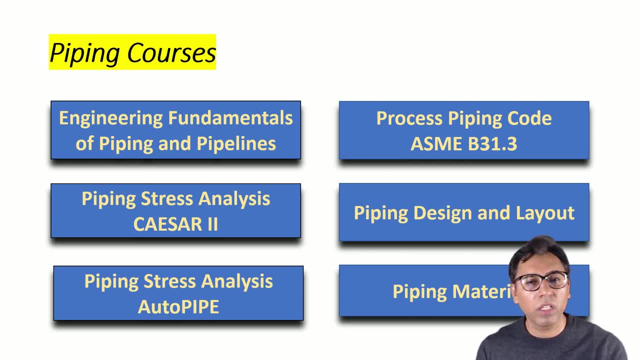 support is more preferable at what location? so there are so much thinking which we need to know and this course will be helpful if you are looking for that information. last course is a about piping materials. so, as I touched base earlier in this course about piping material, so this course will go in more. 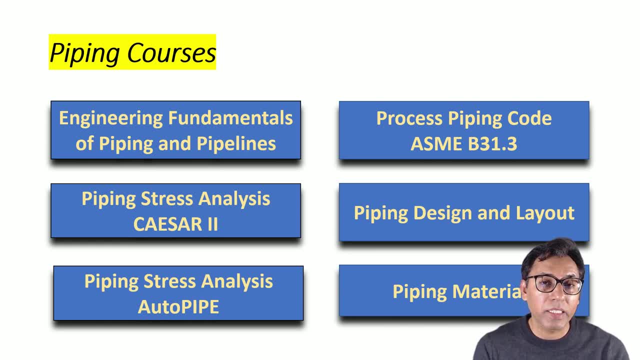 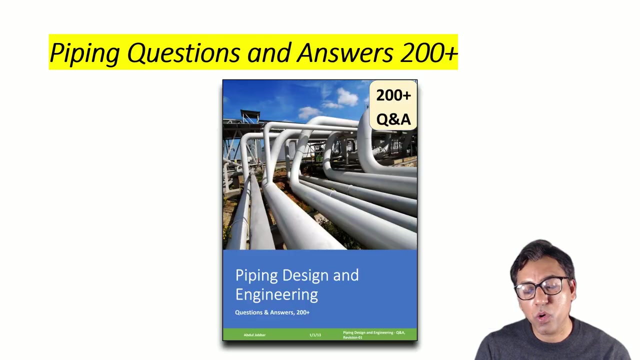 details about what are the applicable standards course in PI about piping components, their materials. they are procurement requirements. this was useful if you want to improve your knowledge about piping material. if you are interested about any course, do get in touch with me and i have already shared my contact details, as i mentioned earlier. um about this, my book, which is a first edition, 200. 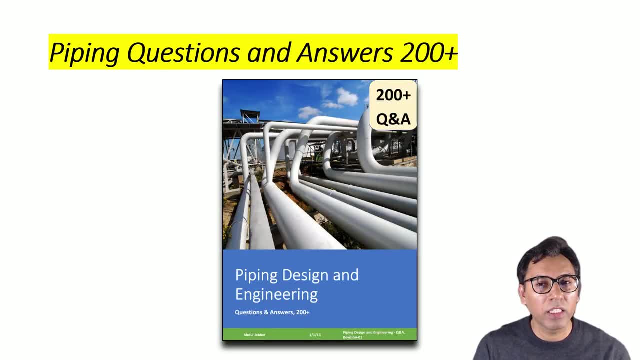 questions, um with answers, and this could gives you a good in-depth knowledge about piping. it's really easy to understand as it is in the form of questions and those questions are from practical experiences people are talk about and you will come across those in your routine projects and rather than just reading boring as like long books of any standard. 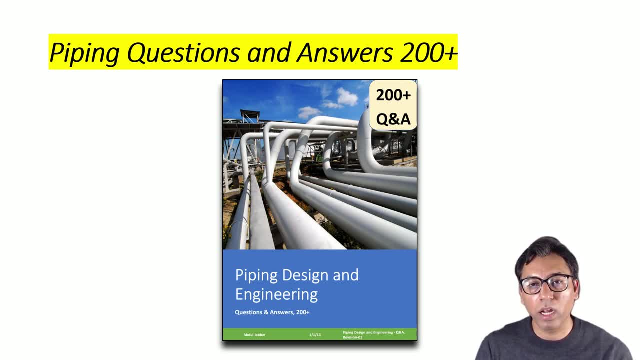 uh, it's really a great idea to grasp all the piping concepts if the real and practical questions are answers. so if you're interested to get that book, so do let me know. and in the last um, here are my contact details as well, so my linkedin page.